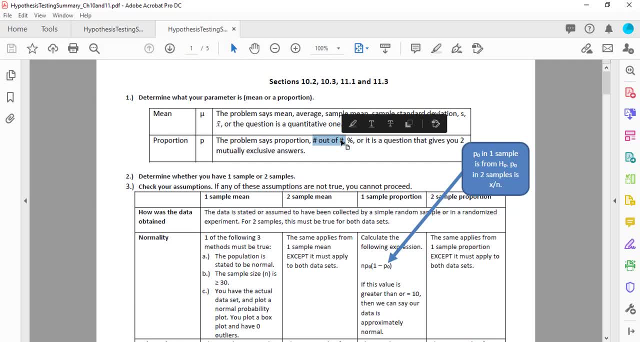 people who smoke out of a total of 105 percentage. They say 36% of students agree with the current percentage Or the question that they ask. it gives you two mutually exclusive answers: Do you agree or do you not agree? Did you vote or did you not? 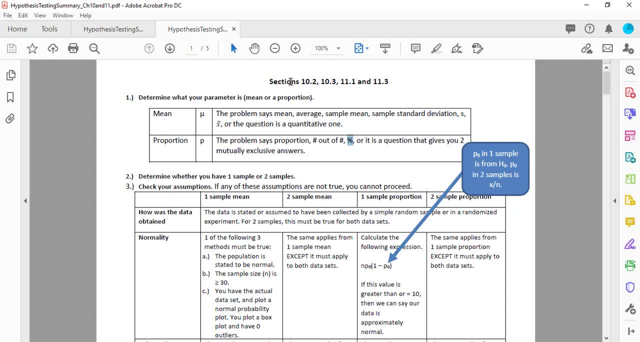 vote. Do you accept what they said or you don't accept what they said? Next, for the problems, you need to determine whether you have one sample or two. So one sample, you're looking at one group of individuals and you're comparing that to a mean or a proportion that's already stated. 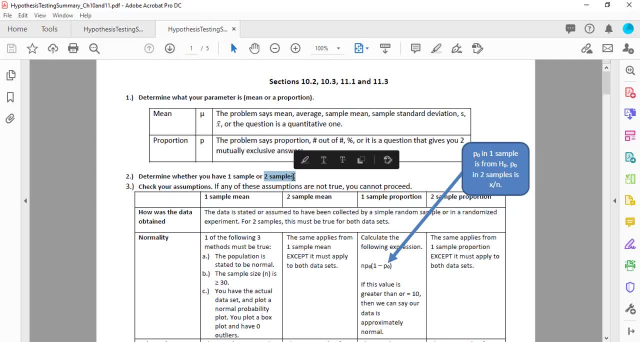 Two samples. you're looking at two groups of individuals and you go in saying at the very beginning that the two groups are the same, So the means are the same, the proportion is the same or the proportions are the same. Next, what we need to do is to check our assumptions. 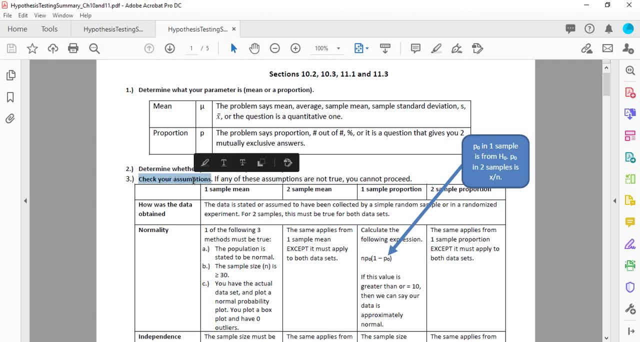 So your assumptions are the items that let you know that you can use this particular process of hypothesis testing. In elementary statistics we focus on something called parametric techniques, where the assumption is always that the shape of the distribution is approximately normal. In other statistics classes the assumption is not made that it's normal, So they use non. 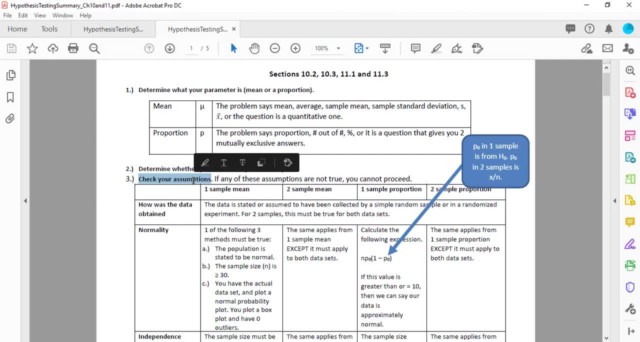 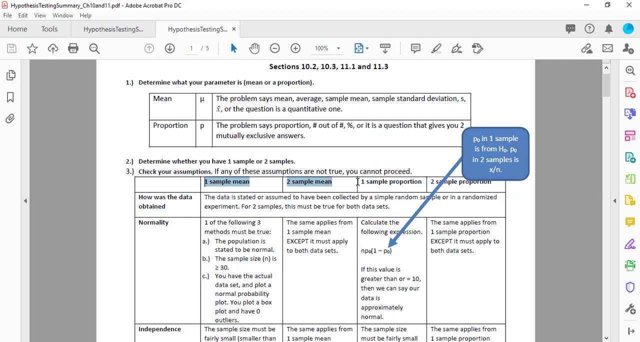 parametric techniques. So if these assumptions are not in place, then we cannot proceed with our types of hypothesis testing. For all of our different methods, whether you have one sample or two, the first thing you always have to do is verify how the data was collected. It should have. 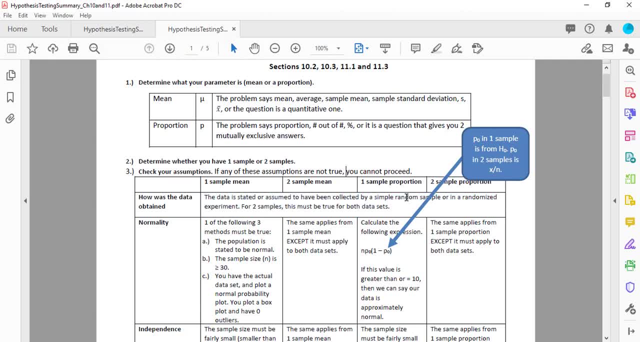 been collected by a simple random sample or in a randomized experiment. If you have both two samples, both of them needed to be collected by simple random sampling. Next, we need to check and make sure that the shape of our distribution is approximately normal, And we have different ways to check for this, depending 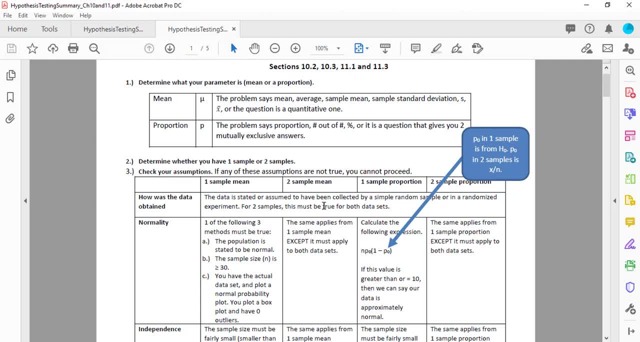 upon whether you have a mean problem or whether you have a proportion problem. That's why that step number one, to make sure you know that if you have a mean problem, one of these three things has to be true. So either in the particular problem, it states specifically that our population 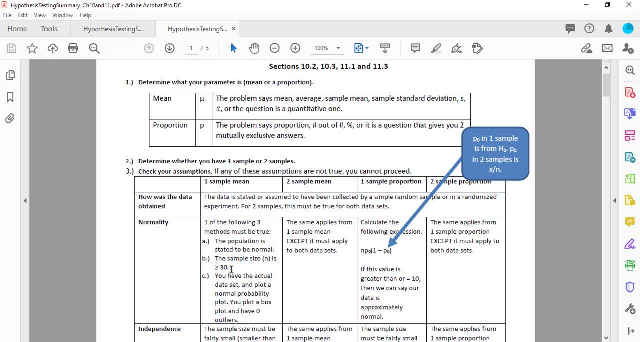 is approximately normal or the central limit theorem says that if your sample size is big enough, it doesn't matter what the shape of your population is, and big enough, according to our textbook, is greater than. if you actually have the data, then you need to plot a normal probability. 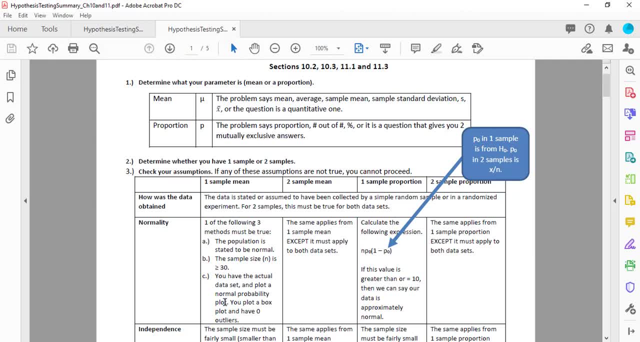 plot and make sure that all of your points are close to that line. you don't have any points that are outside. You also want to make sure that you put out a box plot and you don't have any outliers. If you have a two sample mean problem. you just need to verify these for both. 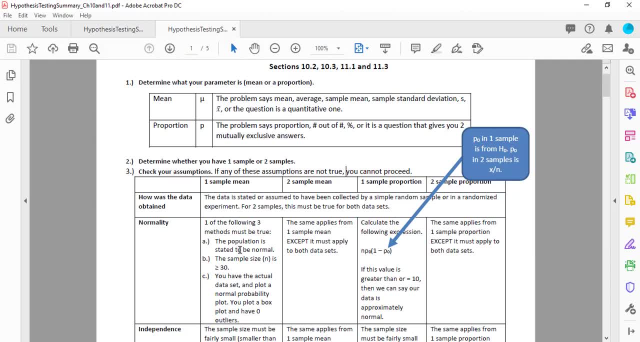 distributions that you have for males and for females, or for people over 40 and for people not under, not over, 40. If you have a proportion problem, the way you check for normality is n times p, times one minus p, And if that value is greater than or equal to 10, then we can say the: 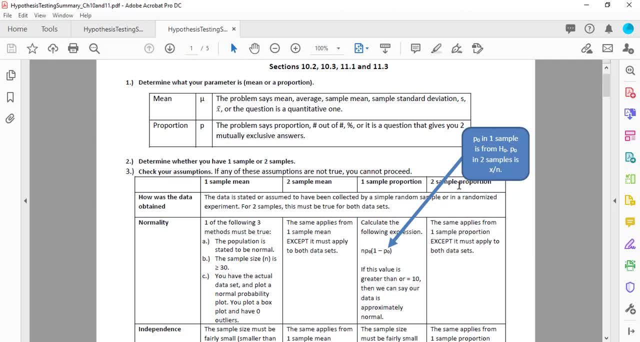 shape of our distribution is approximately normal. So if you have a two sample, mean problem, you just need to verify these for both distributions that you have. If you have a two sample mean problem, you're using the actual proportions. So you'll do one for one, the first group. 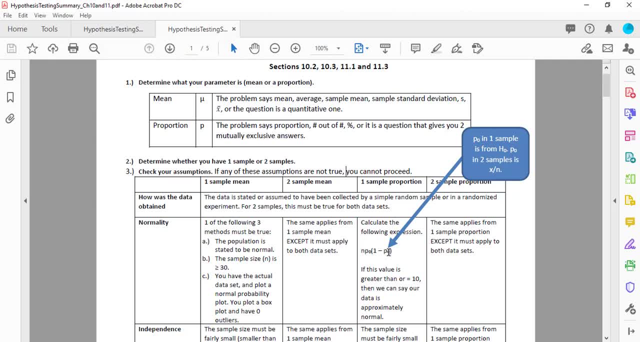 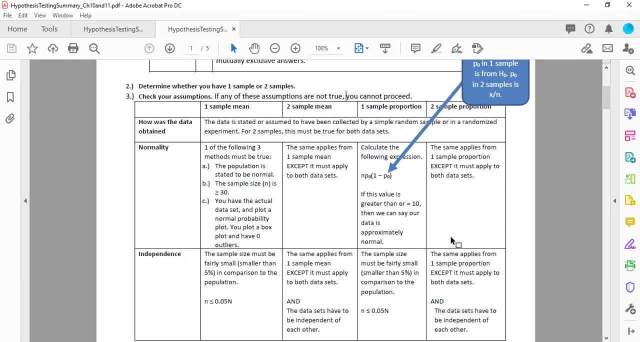 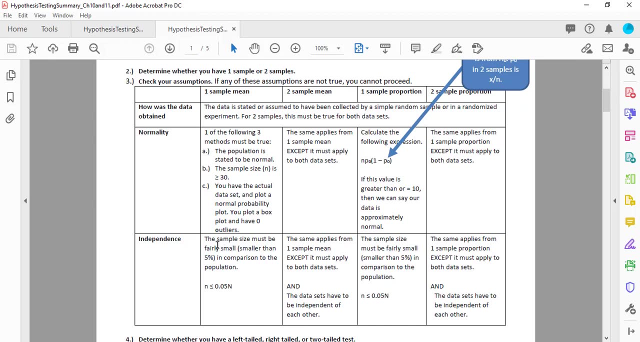 you'll do one for the second group, and the proportions you're using are the sample proportions. So that's the difference between these two. You must also have independence in all of your samples. Independence means that, well, part of it means that when we are doing 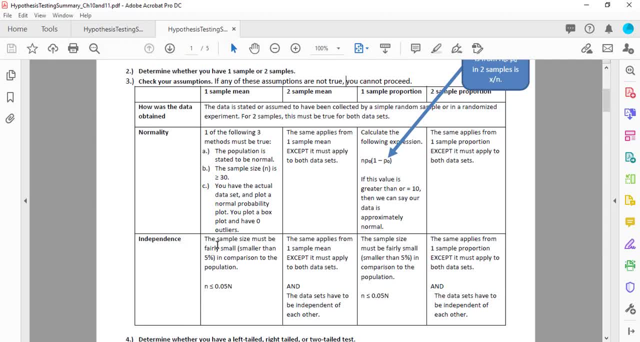 this sampling distribution. when we're taking all of these samples, it's okay for us to have multiple individuals in different samples. So the way we say that that's okay is we make sure that our sample size is less than or equal to five percent of the population size. If you have two. 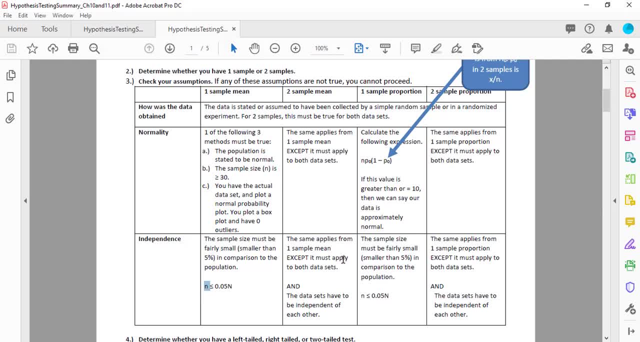 samples. you need to check that for both of your samples, both of your groups that you're studying, and you want to make sure that your groups are independent of each other. So if you're comparing male and female, you're going to want to make sure that you're comparing male and female. So if you're 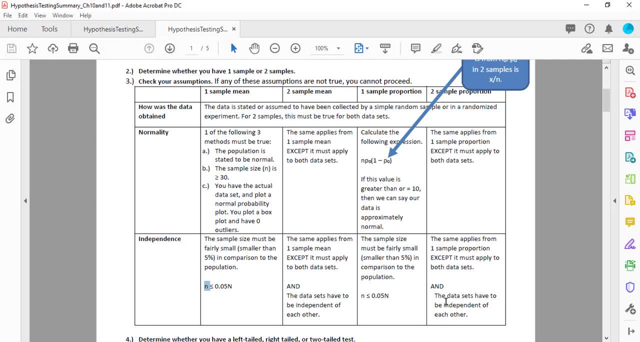 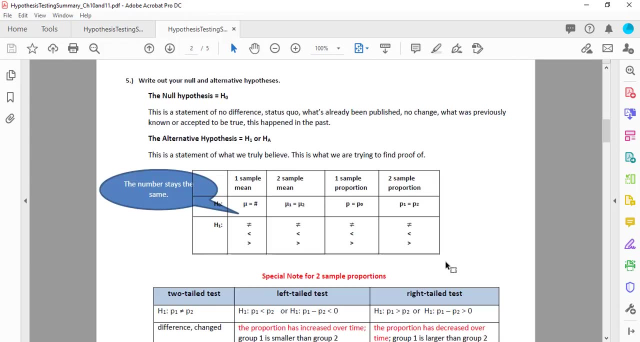 comparing females, you're only in the male group or you're only in the female group. You cannot have an overlap there- Or your age- you're either over 40 or you're not over 40. So there's no overlap in any of either of these groups. Once you've verified your assumptions, we need to determine. 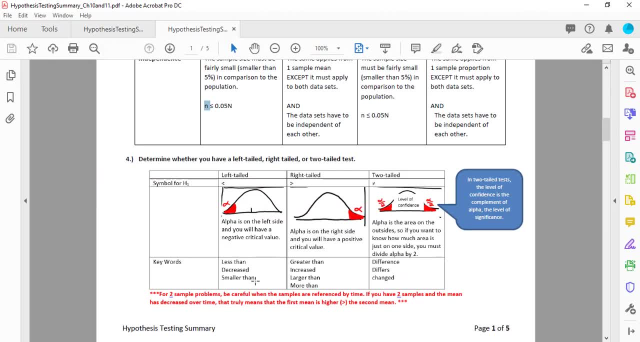 what type tail test we have, and your keywords are what you're going to pay attention to. So less than, decrease or smaller than means you have a left tail test. The symbol that you're going to use in your alternative hypothesis is less than, and when you're graphing this for the classical. 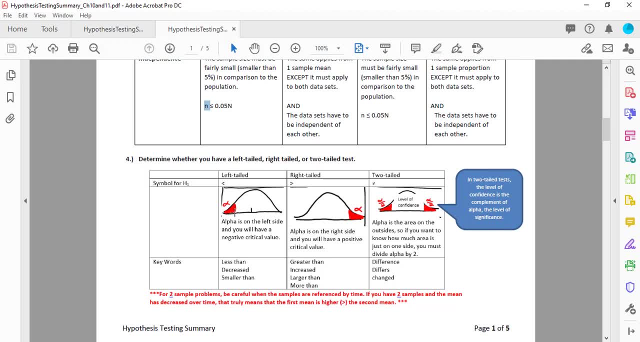 approach. this tells you that alpha is on your left hand side, So your critical value is going to end up being negative. If your keywords are greater than, increased by larger than or more than, then you have a right tail test. That means for your alternative hypothesis: 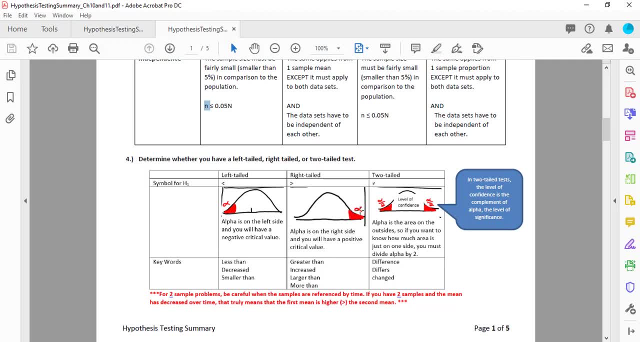 you're using a greater than sign. That means that alpha is on the right and you're going to have a positive critical value here. If you have a two tailed test, your keywords are: is there a difference between the groups? do the groups differ? have the value changed and so your 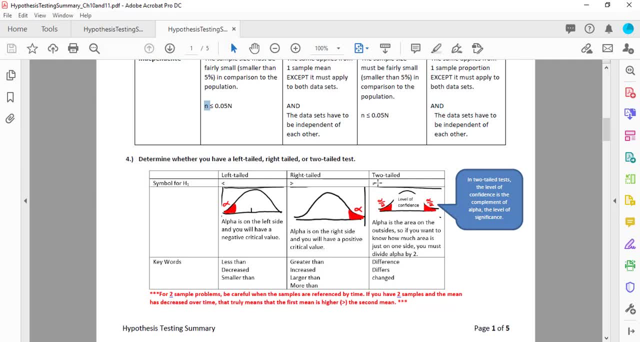 symbol that you're going to be using here is not equal to, And you're going to have two critical values. You're going to have a negative z or t sub alpha over 2.. You're also going to have a positive z or t sub alpha over 2.. For two tail tests: your level of confidence. 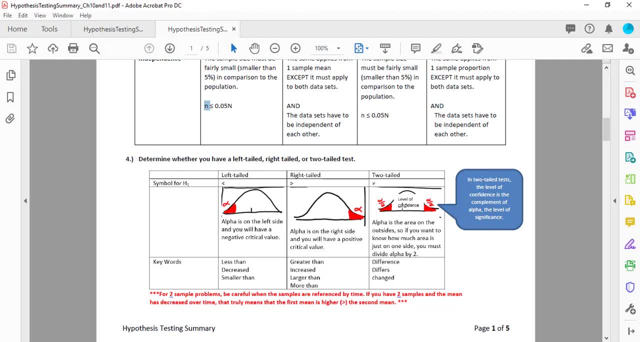 is the complement of alpha. Your level of complement is the complement: 1 minus alpha gives you your level of confidence, and vice versa, 1 minus your level of confidence, as a decimal of course. so if you have the 99th percentile, this is 0.99,. 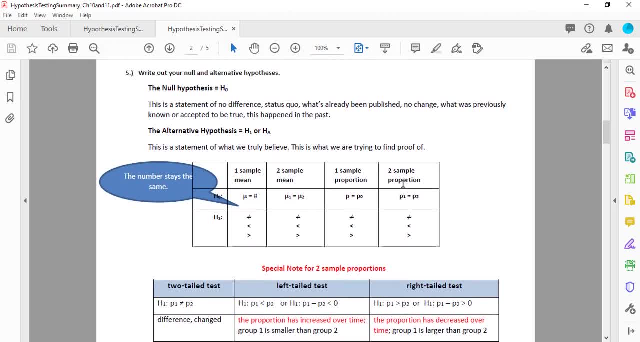 then that will equal to your alpha. After that, write out your null and alternative hypotheses. Your null hypothesis is always your control. your statement of no difference. It's already been published. It's something that hasn't changed. This is your baseline group. This is what you would think of, kind of like. 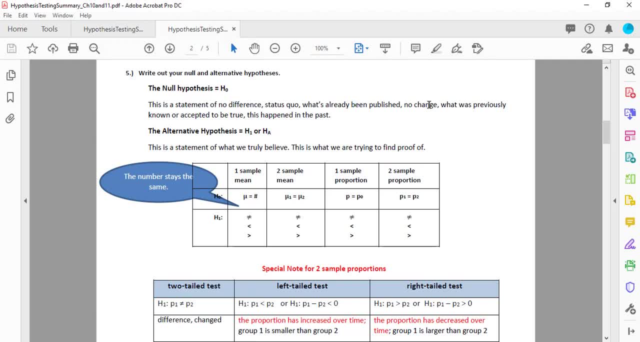 an experimental design, your control group. So it's what you've always done. what's already been published, what's already established, is no different from what you've already done in the past. H1 or HA is your alternative hypothesis. This is what you're trying to find proof of. This is what 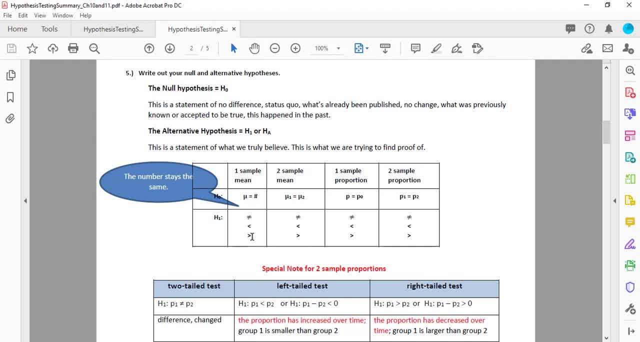 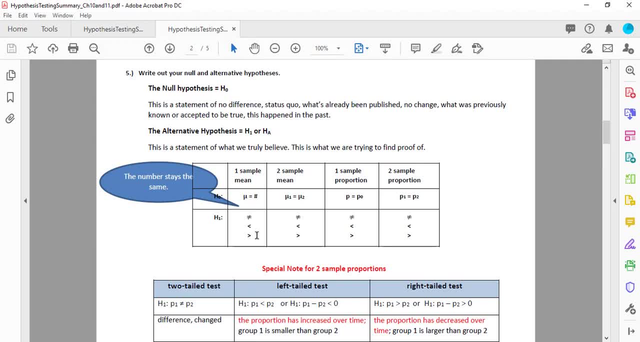 What you need to remember is that here the numbers that you have for one samples are going to stay the same. You're not going to change those For two samples. you always go in saying your null is always that these two groups are the exact same, They're equal to each other. 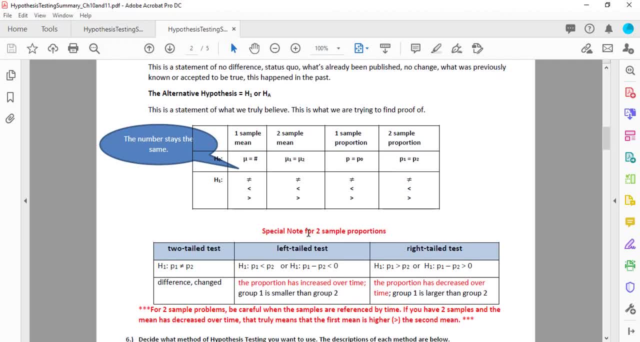 And I have some special notes in red for you about two sample proportions. So one note is you can write two samples two different ways, So you can leave both of the symbols on both sides or you can move the symbol to the other side. So for here it's just imagine if we solve this. 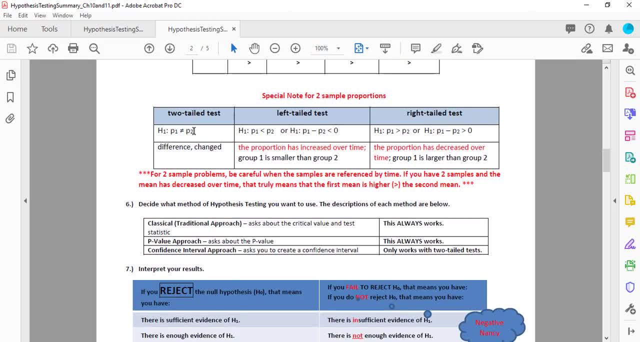 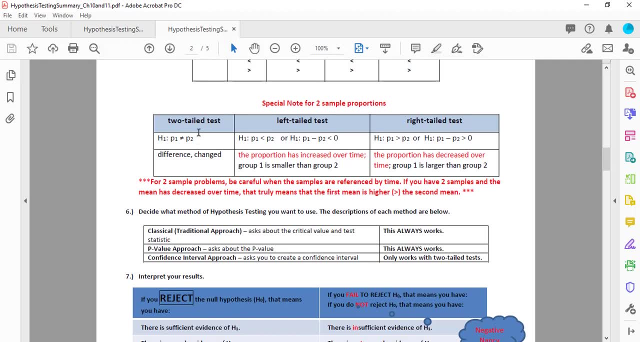 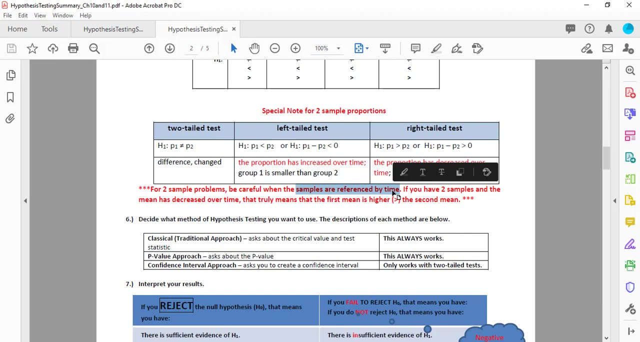 So this is P sub one minus P sub two is not equal to zero, So it just depends on your software that you're using and how it's going to be written out. Also, another note is to be careful. Are you able to calculate your value based upon the application of the problem? If you're talking about 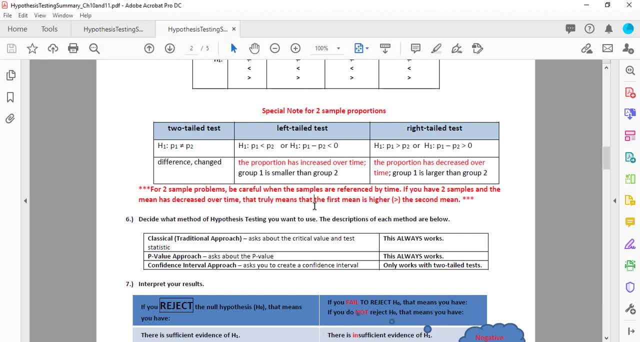 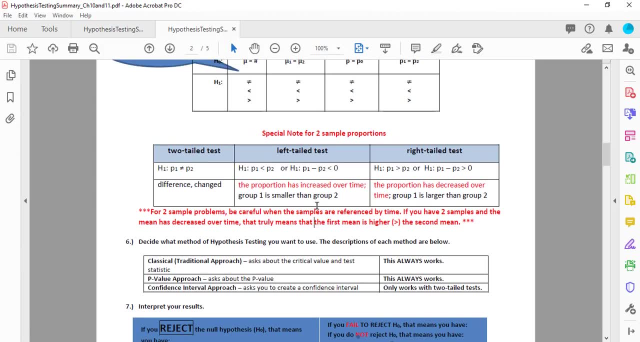 differences in time, then your symbols are going to be backwards. And what I mean by that? if you're comparing like 1970 to 1980, if you say the value has decreased over time, you would initially go into thinking that that decrease. 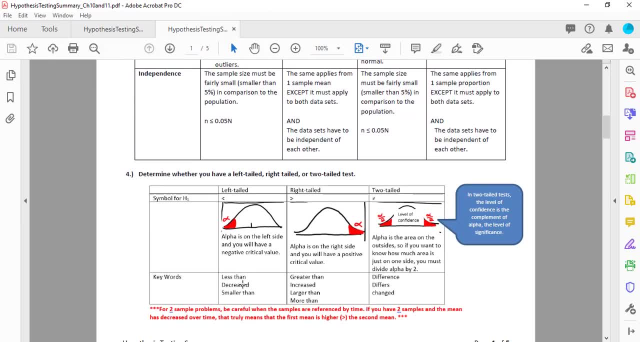 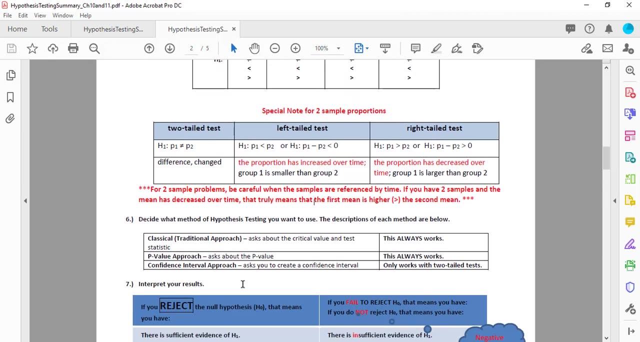 Is less than the problem with. that is 1970.. If your value has decreased over time, This means that your value will decrease over time. in 1980 that really means in 1970 the value is greater. so be careful about those types of problems. next you decide on which type of hypothesis. 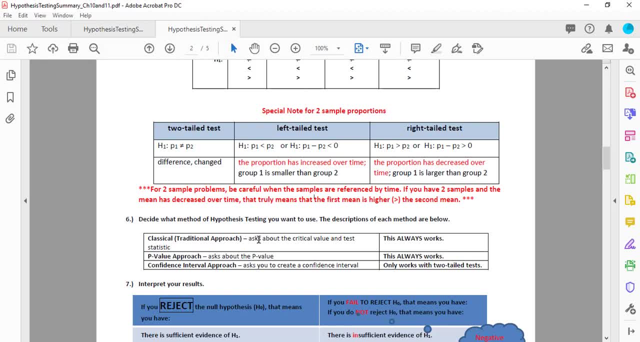 testing method you want to use. your classical approach is going to always ask you about a critical value in a test statistic. this method always works, no matter what kind of problem you have- left tail, right tail or two tail, you have your p-value approach. that's all. it's going to ask you about a p-value. 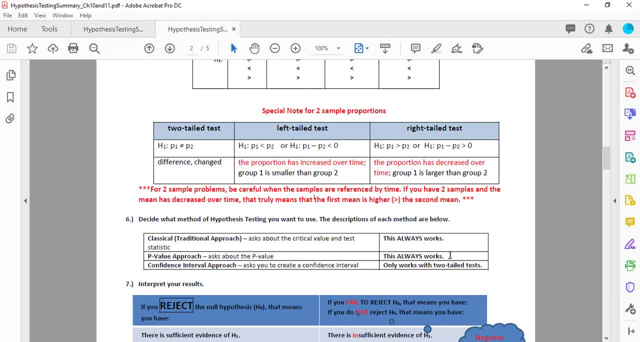 this method always works as well, and the method we're talking about in this video is the confidence interval approach. it only works with two tail tests, so you always have to have those keywords of: are the values different? have the values changed? then we interpret our results after that, so we reject the null. 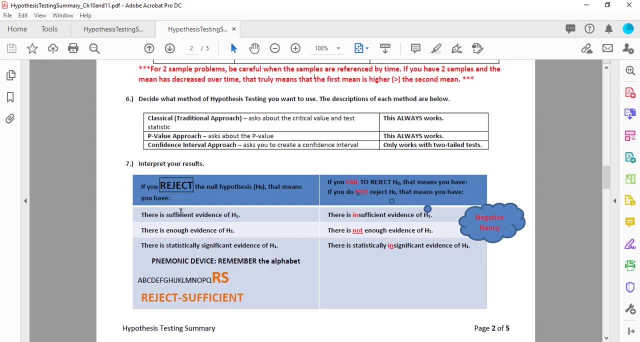 hypothesis and the reason why we reject is because there is no null hypothesis. and the reason why we reject is because there is no sufficient evidence. or we can say there's enough evidence or we can say there's statistically significant evidence of the alternative. so you reject the null because you have enough proof of the alternative and your 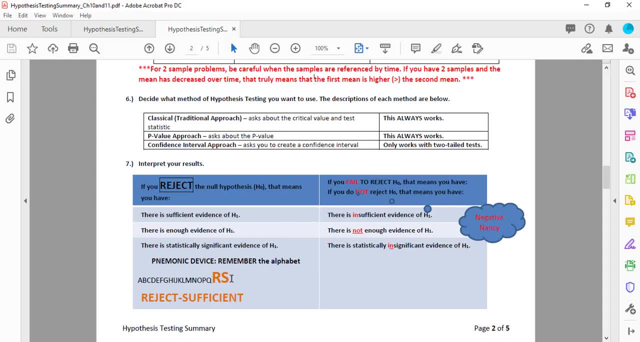 mnemonic device RS. if you reject it is because there's sufficient evidence. then you can fail to reject. so that means you don't get rid of the null hypothesis, and you don't get rid of the null hypothesis because you don't have enough evidence of the alternative. so your mnemonic device here negative. Nancy, you have fail. 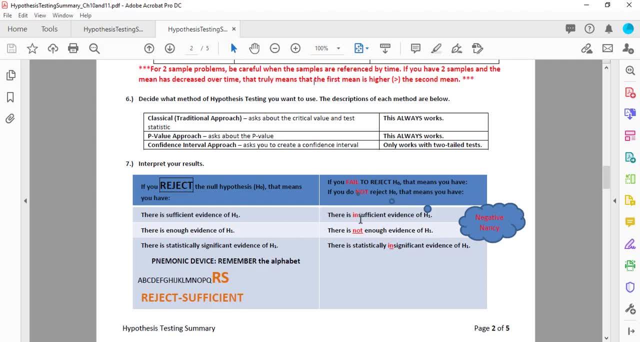 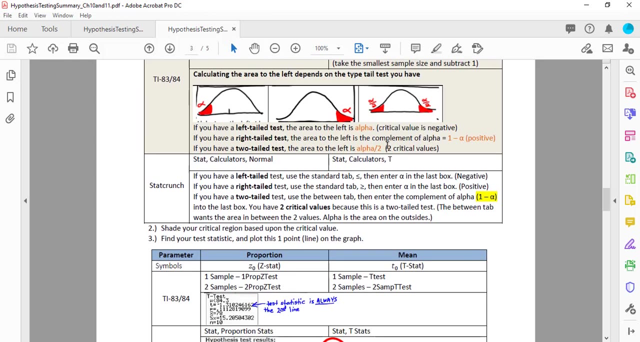 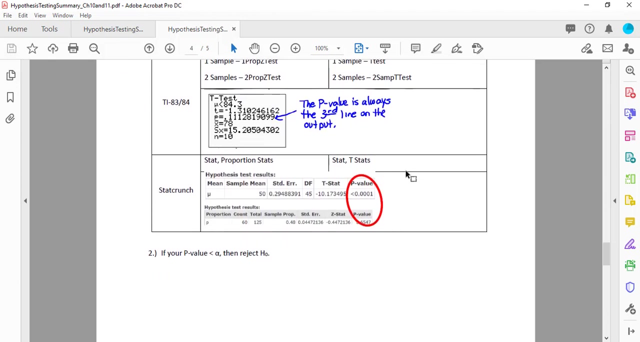 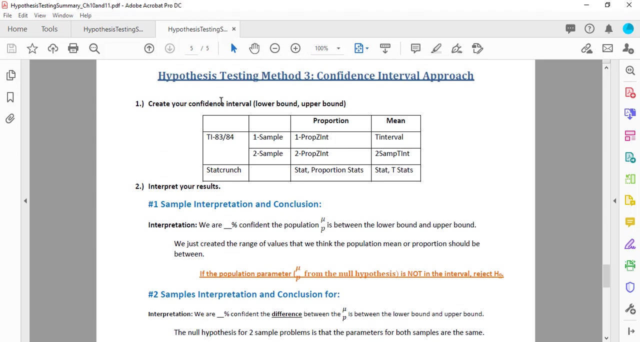 and insufficient or not and not, or fail and not, so those prefixes for in gives you a negative connotation there. then you have classical approach, which we covered two videos back. you have p-value approach, which was one video back, and now confidence interval approach. so once again, you only can use the confidence. 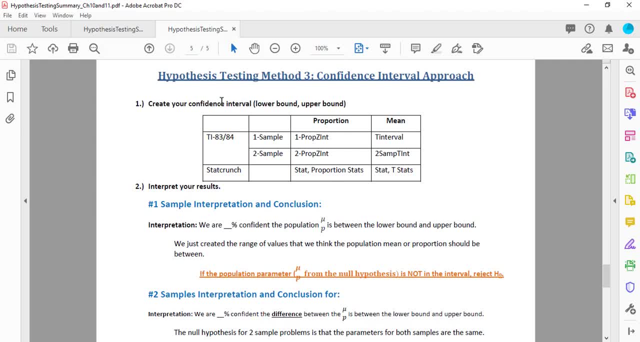 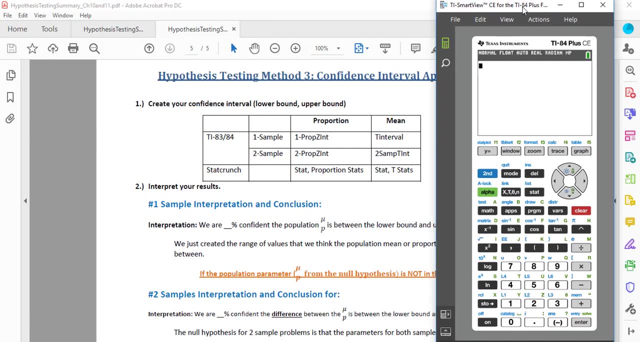 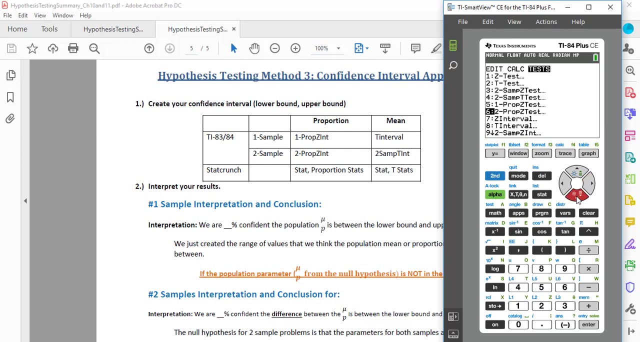 interval approach. when you have a two-tailed test, you need to create your confidence interval. if you are a graphing calculator person, then where you are going is under stat, you're going under test and then, just like we did in chapter nine, T interval is when you 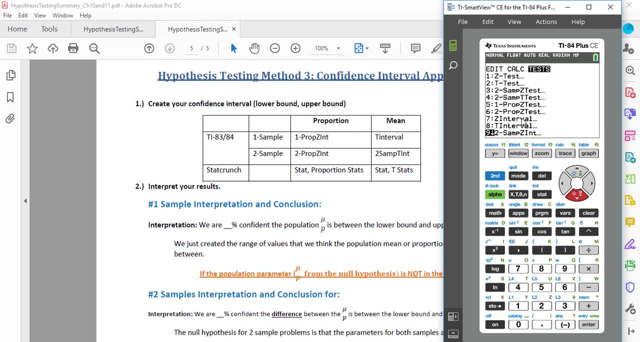 have a one sample mean problem. Two-samp t int is when you have a two sample mean problem. So in our elementary statistics class our assumption is always that we don't know what the population standard deviation is and we use the sample values. and since we do that we're working with the t distribution. So t. 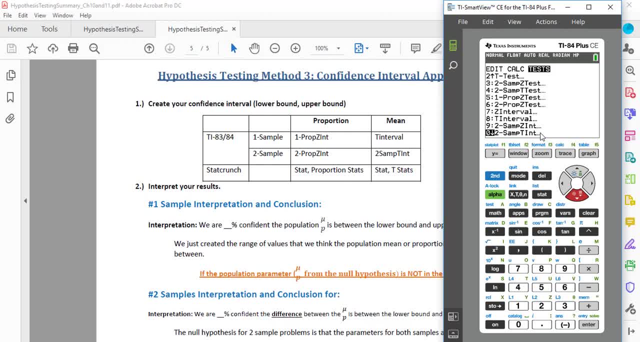 interval and two-samp t int. If we have a one sample proportion problem, we're going under one-prop z int. If we have a two sample proportion problem, we're going under two. I'm sorry, two-prop z int, One-prop z int and two-prop z int. If 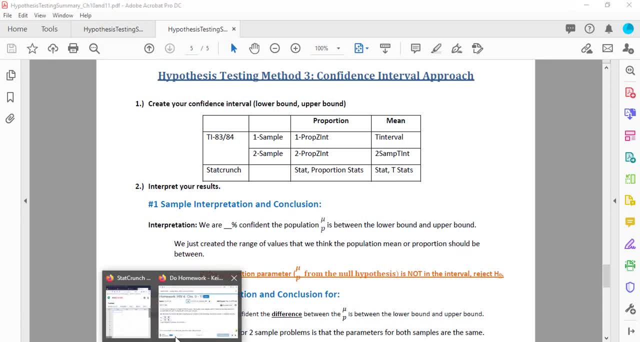 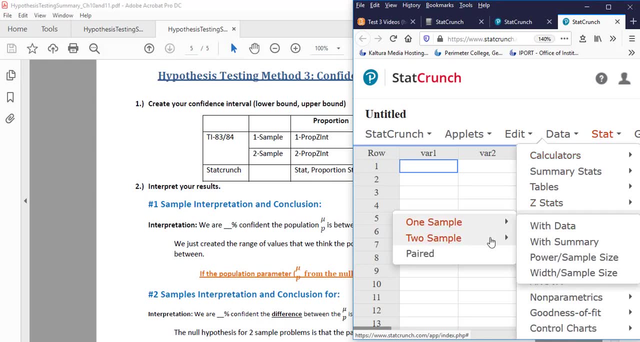 you're a stat crunch person, then you're under stat and t stat- One sample or two. we no longer do paired in this course. or you're under proportion stats and then one sample or two. We interpret our results and we did this in chapter nine. 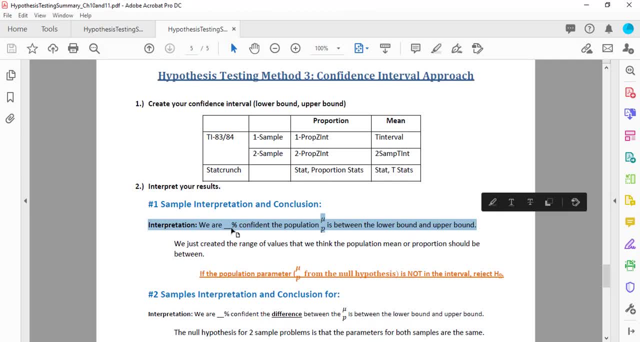 We say that we are blank confident, percent confident. so 95%, 99% or 90%, typically, Confident that the population mean- if it's a mean problem, or the population proportion- if it's a proportion problem is between the lower bound and the upper bound, the smaller number and the bigger number. 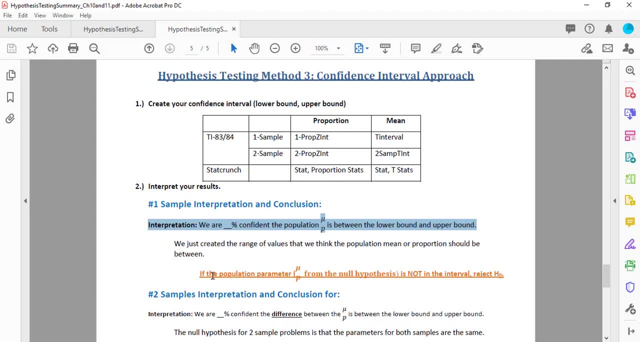 So the way we interpret this for hypothesis testing is that if the population mean or proportion from the null hypothesis is not inside of that interval, that's when we're going to reject the null hypothesis. So your null hypothesis is your baseline value, what we assume to be true. 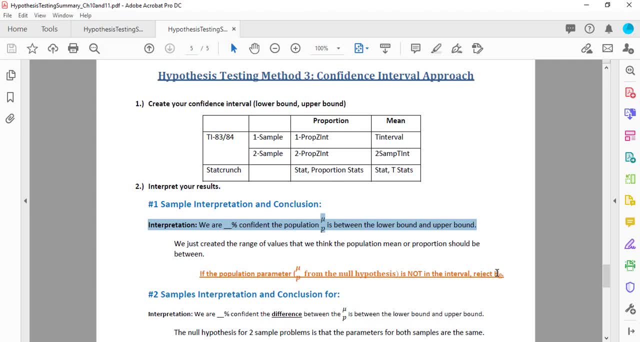 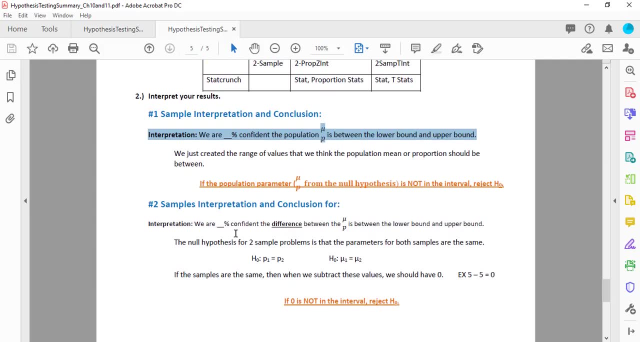 If the interval that we create based on our sample doesn't say that that number is possible, then that's when we reject the null hypothesis. Two samples. our interpretation is: we are blank percent confident, 90,, 95, or 99, that 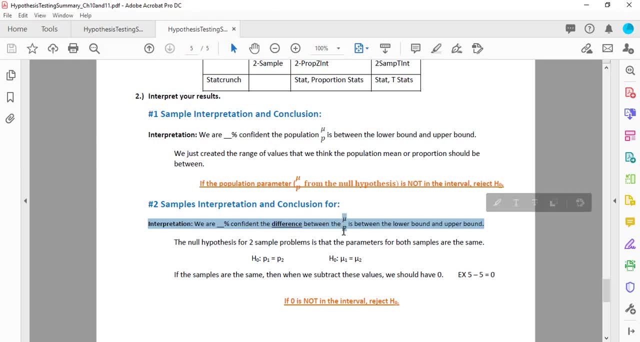 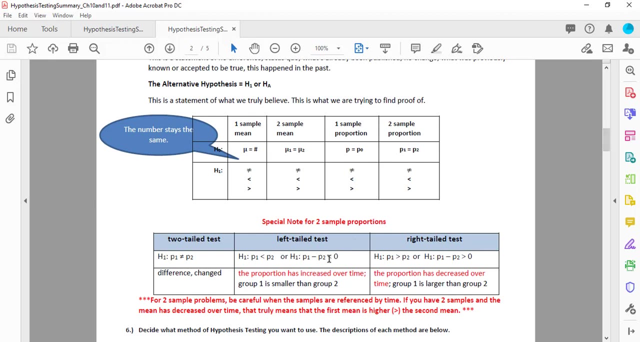 the difference between the means or proportions is between the lower bound and upper bound. So for two samples, we're always looking at the difference, We're subtracting them and that's why you have two different ways of writing your null answer, An alternative hypothesis. in here you're supposed to also have p sub one minus p sub. 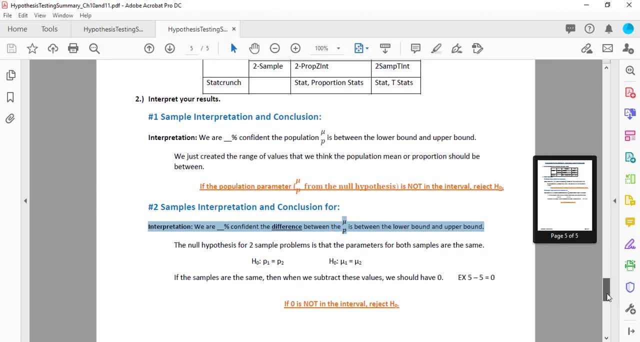 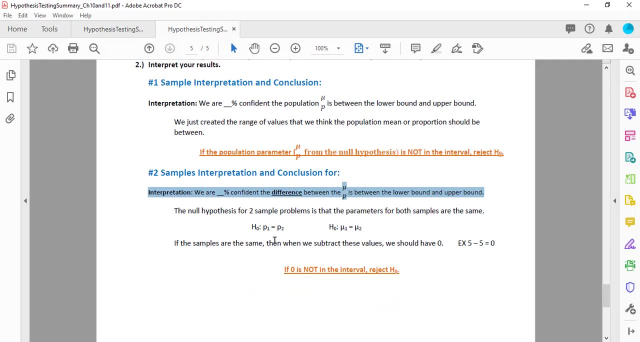 two is not equal to zero as well. So when you're subtracting two values that are the same, when you subtract them, you should get zero if they're the same. An example: five minus five or 10 minus 10, or 1,000 minus 1,000, or 0.4 minus 0.4.. 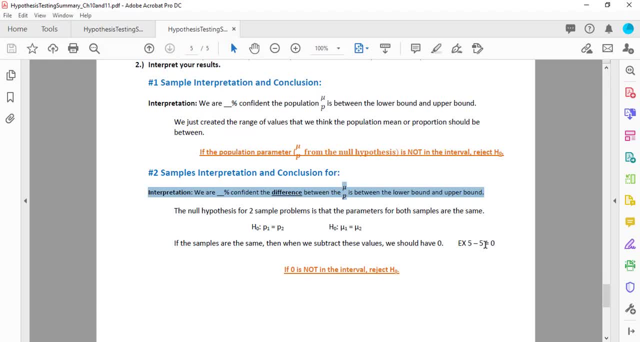 If we go insane that these two samples are the exact same, When you subtract them, you're supposed to get zero. So for two samples, the way you complete hypothesis testing is that if zero is not in your interval, if zero is not between your lower bound and your upper bound, that's when we're going. 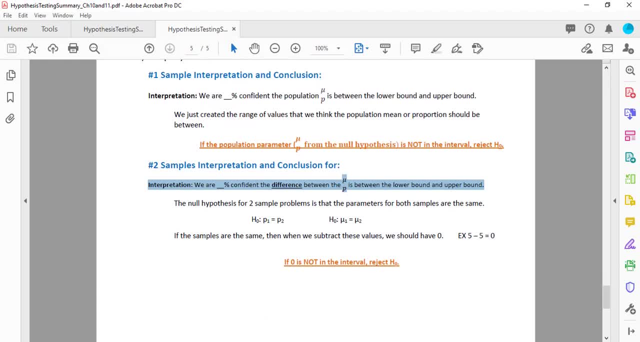 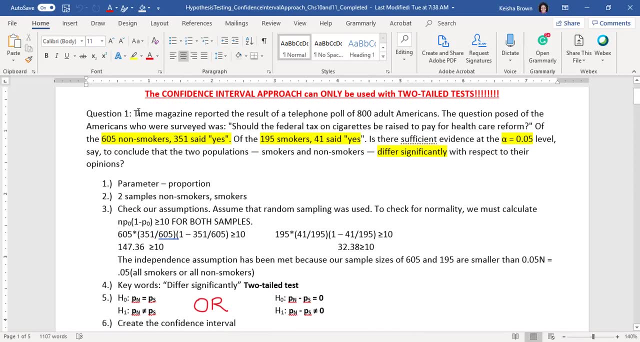 to reject the null hypothesis. Now let's look at your completed lecture notes. Question number one: Time Magazine reported that the result of a telephone poll of 800 adult Americans. The question posed to the Americans was: should the federal tax on cigarettes be raised to? 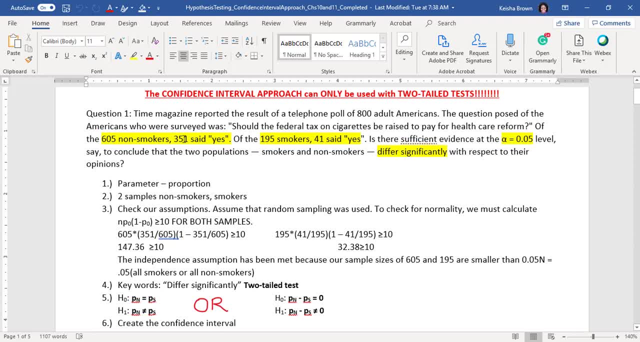 pay for health care reform. Of 605 non-smokers, 351 said yes. Of the 195 smokers, 41 said yes. Is there sufficient evidence at the alpha equals 0.05 level, say, to conclude that the two populations, smokers and non-smokers, differ significantly with respect to their 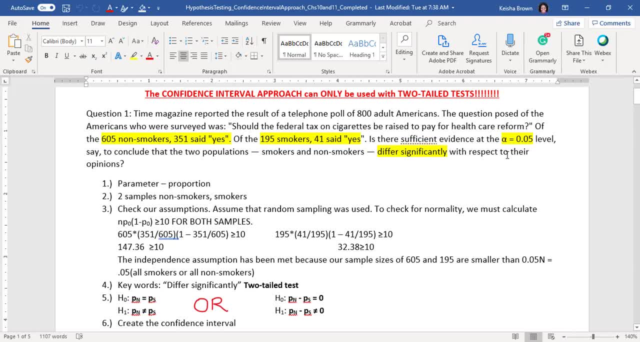 opinions. So for all of these problems, you need to read them. Pull out the key information that you need. First key information is that you have two samples: You're looking at non-smokers and you're looking at smokers. Next, you need to make sure you know that this is a proportion problem because of the type. 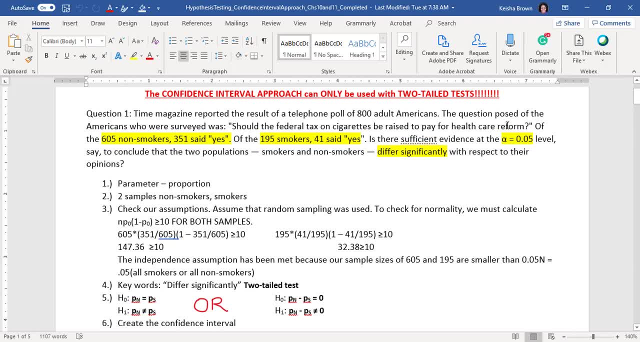 of question that's asked: should taxes be raised? You're either going to say yes, they should, or no, they shouldn't. So that's one way. you know it's a proportion problem. You also know it's a proportion problem because you have a number out of 100.. 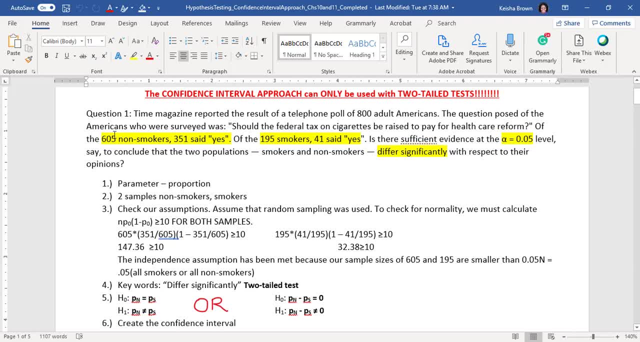 You're going to say yes to one number out of another number. 351 said yes out of a total of 605.. Then you need to always check your assumptions. When you have two samples, you need to check your assumptions for both groups. 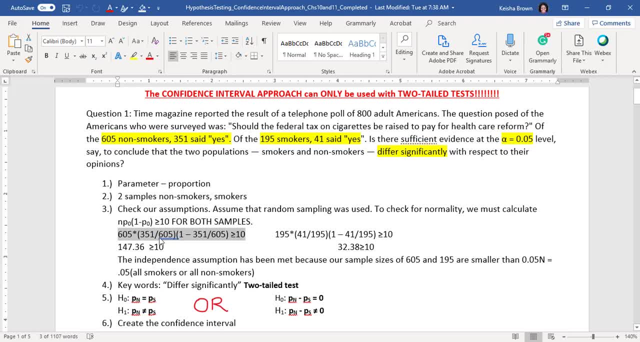 You need to check your assumption for non-smokers and making sure that your p-value you're using is your proportion, your sample proportion here, So that should be p-hat, And then you need to check it for your other sample, For smokers as well. 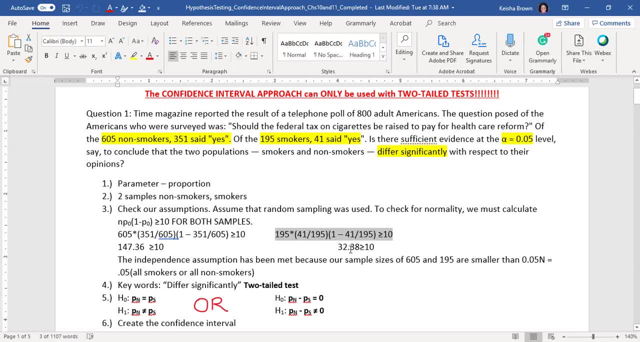 And if that value is greater than or equal to 10,, then the shape of your distribution is approximately normal. Your third assumption is independence. We're pretty sure that they are. more than 5% of the population is bigger than 605.. And same thing, 5% of the population of smokers is going to be a lot larger than 195.. 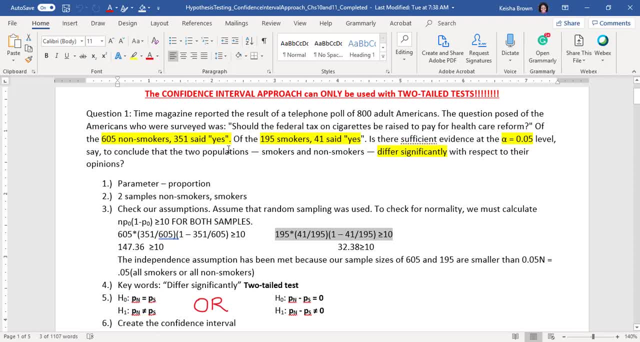 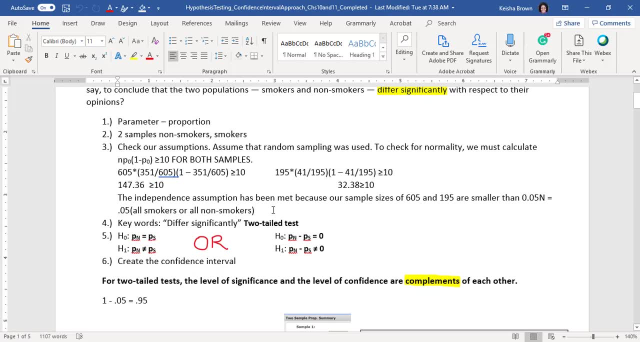 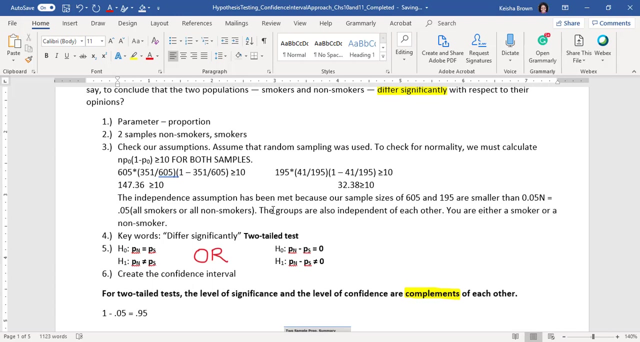 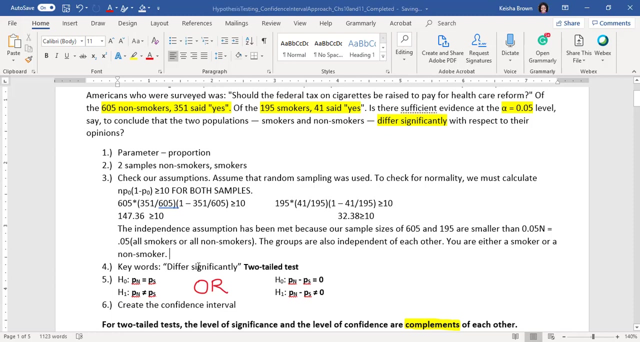 These groups are also independent of each other. You're either a smoker Or you're not a smoker, One or the other. Number four Key words to let you know what type tailed test you have is that it says: differ significantly. So you know you have a two tailed test. 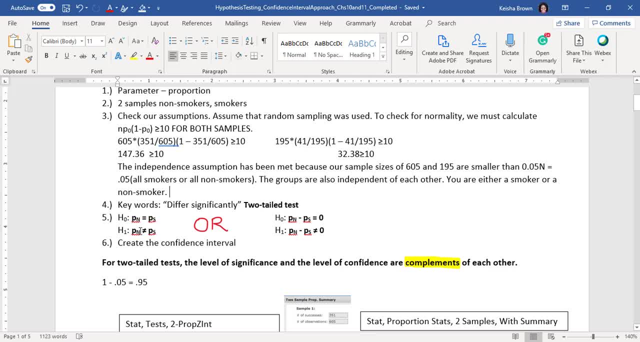 You can write your null. You don't have to write your goal. That's what you need to learn in order to get a final answer. You want to start off as a smoker, you want to finish 2 samples and then we're going. 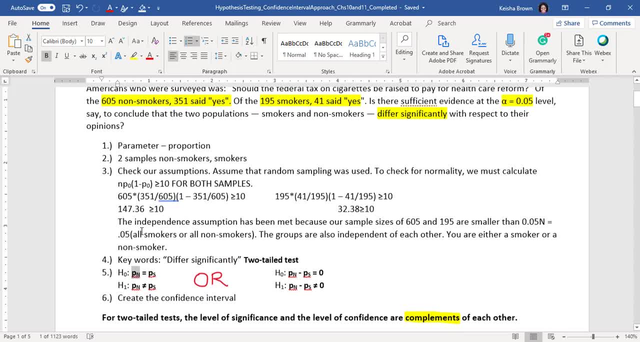 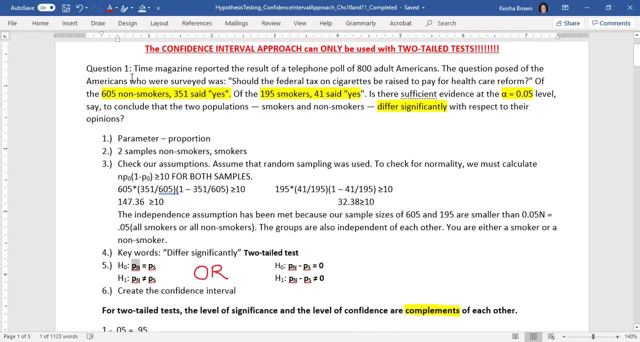 to build an alternative hypothesis, Two different ways. We are putting p sub n first, because that's what they talked about in the problem. first Non-smokers. So for two samples, whatever group is listed first, that's going to be the symbol that you 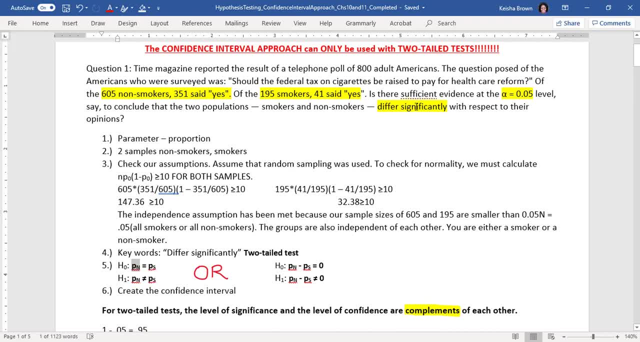 used first. Our alternative hypothesis is that they differ significantly. So you can set it to zero or you can set them to each other. Your null hypothesis is that you always go in saying that these groups are the same. So you can set it to zero or you can set them to each other. 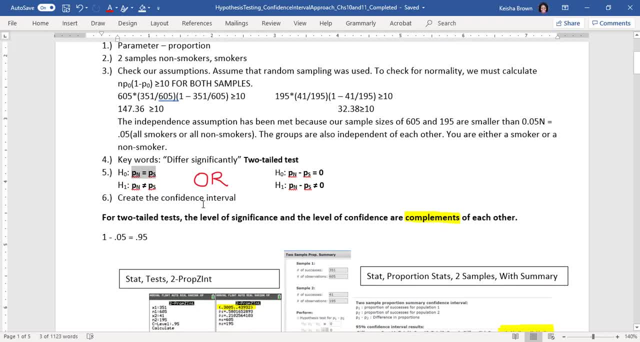 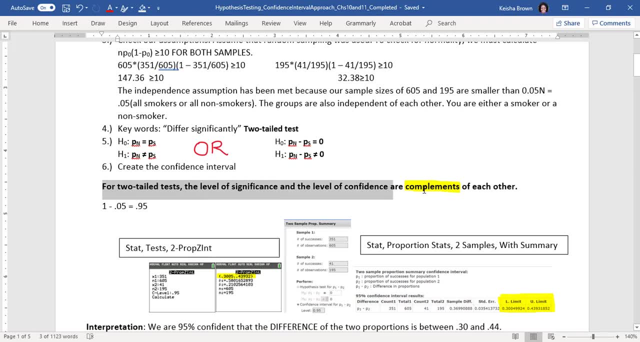 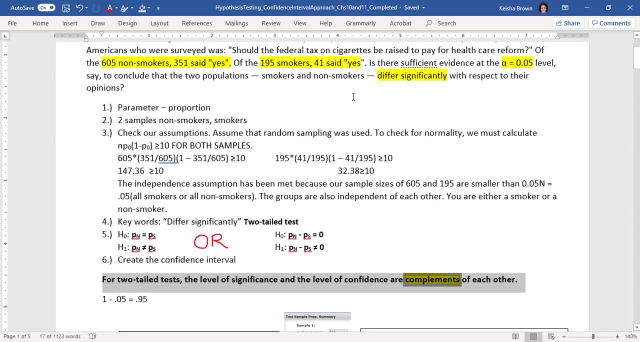 Your null hypothesis is that you always go in and say that these groups are the same. now we create our confidence interval. remember that for two-tailed tests, the level of significance and the level of confidence are complements of each other. so in this problem, they told us to use alpha equals point zero five, since it's 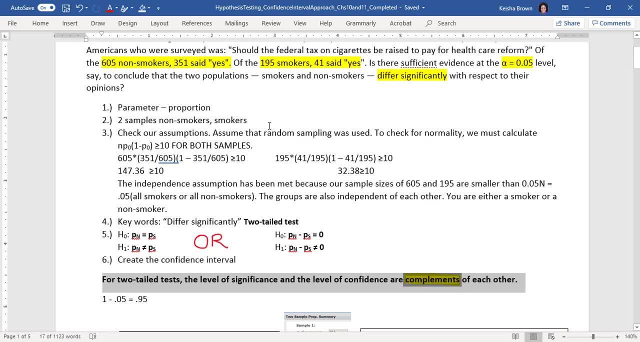 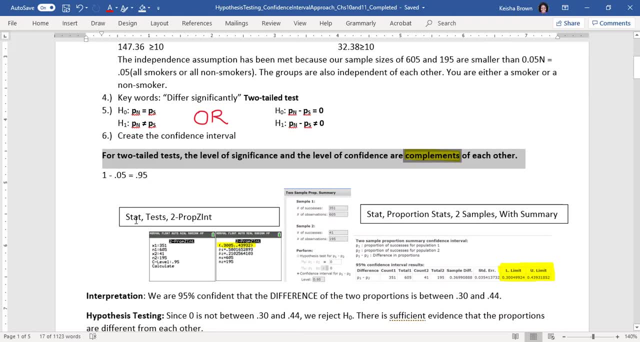 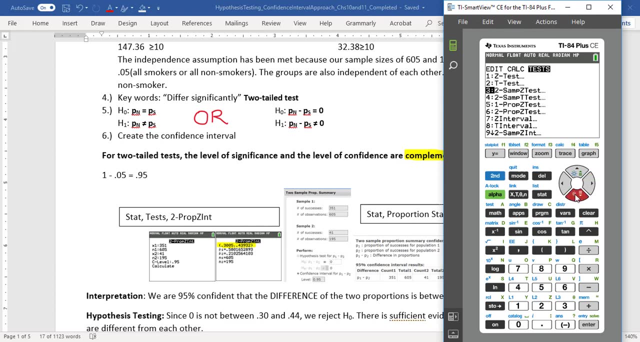 a two-tailed test. that means alphas on outsides, it's split over the outsides. so our level of confidence is point nine five. so if you're a calculator person, you're going under stat, you're going under tests, you're going under to prop. 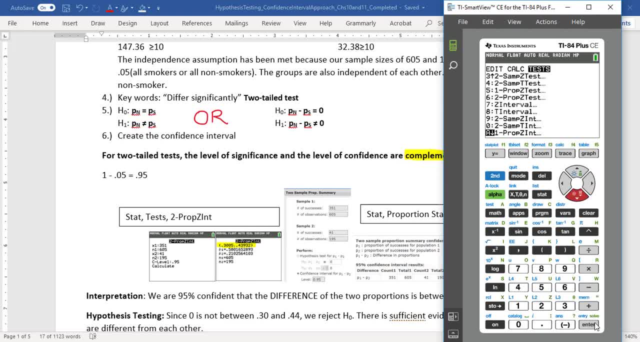 z-int and I selected one and not two. then x sub 1 is whatever group they talked about first. first he talked about non smokers except to. they talked about non-smokers except to. they talked about non-smokers except to. they talked about smokers. C level is our level of confidence, our complement of alpha and 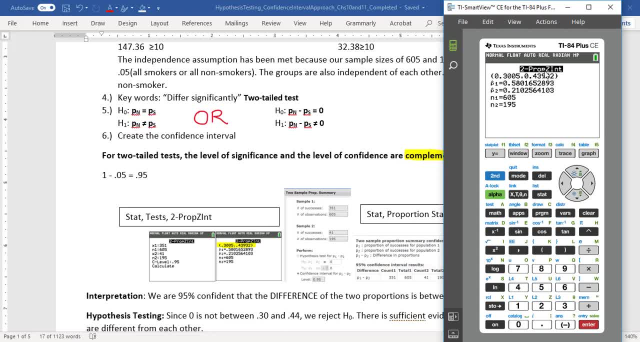 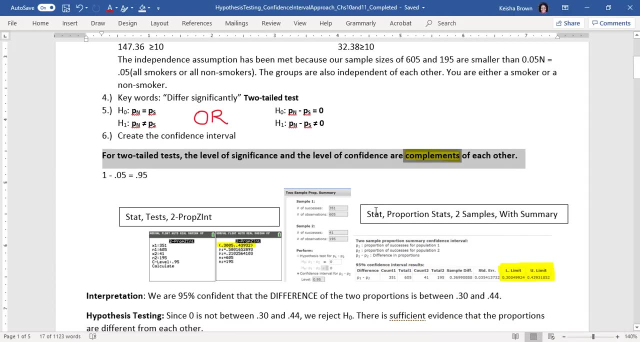 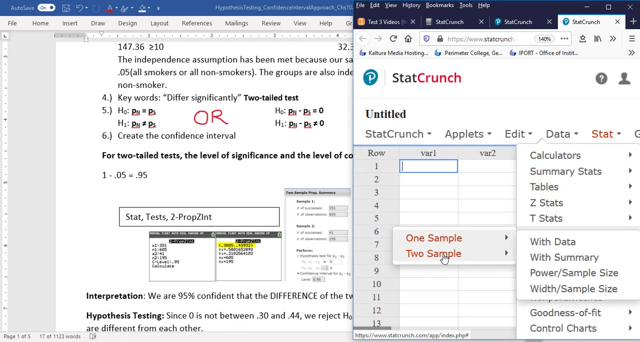 when we press calculate, there is our interval. so we interpret this by saying we're 95% confident that the difference in opinions of the non-smokers and smokers is between point three and point four. four: if you're a stack crunch person, you're going under stat. you're going under proportion stats. we have two. 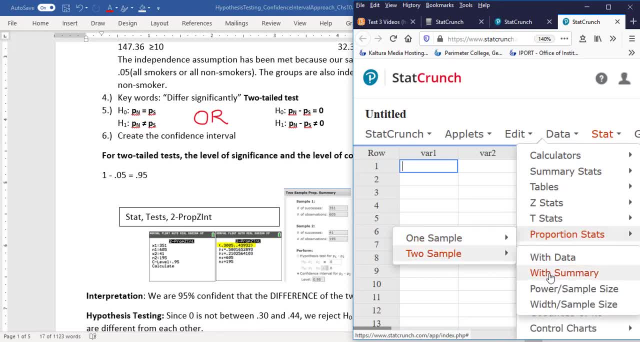 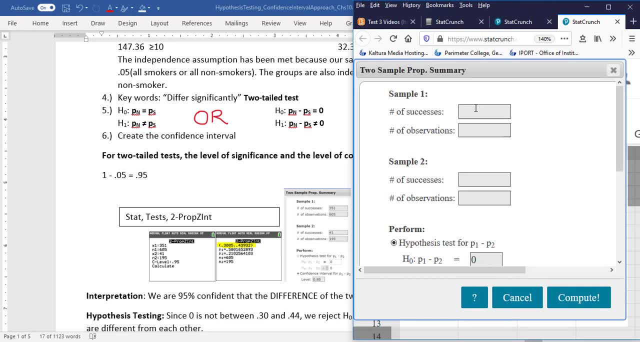 samples. you have summary information because they told us 195 out of this other number. well, 41 out of 195, sample number one is whoever they talked about in the problem first sample. number two is whoever they talked about second. we're doing hypothesis testing, so we want to make sure that we're doing hypothesis. 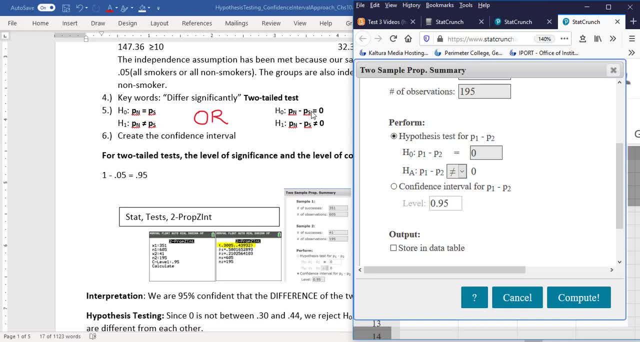 want that first radial button and in stack crunch they do write it in this second form where you set it to zero, and This is a two tailed test. so we want not equal to well. this first part, I'm sorry, is what you would do if you're. 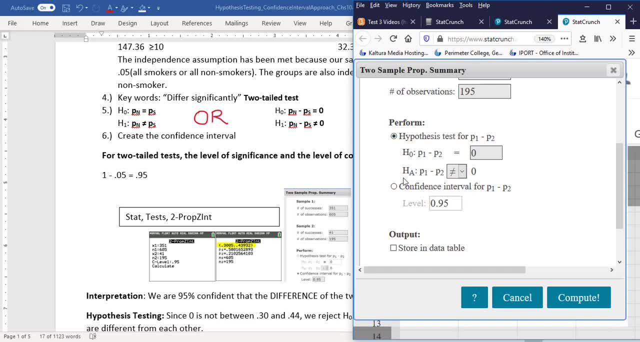 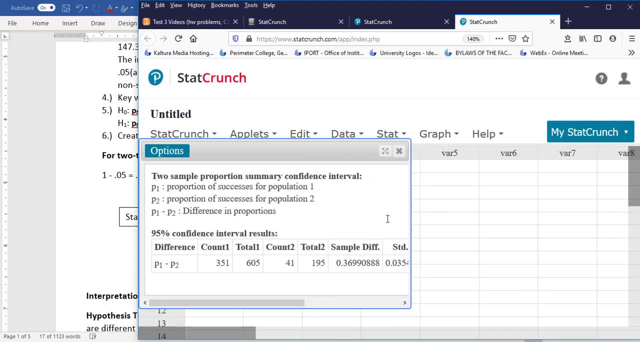 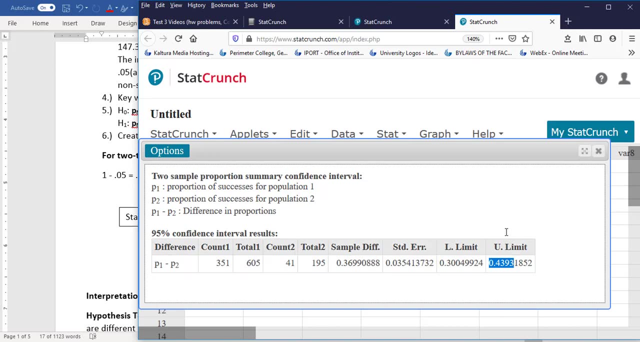 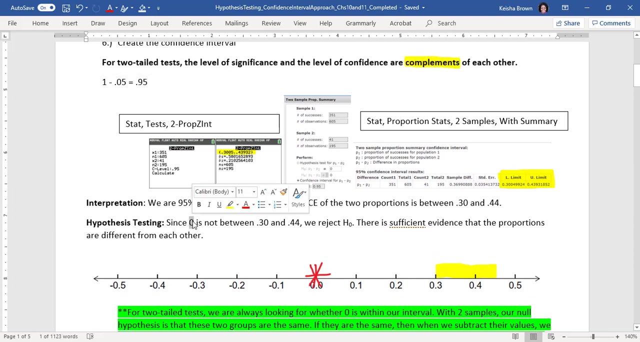 doing p-value approach or classical approach. we actually want the confidence interval and compute and when we expand this table, lower limit is your lower bound, upper limit is your upper bound. So, hypothesis testing, since zero- remember, for two sample proportions- we're looking for is zero between your interval is not between 0.3 and 0.44, we're going to reject. 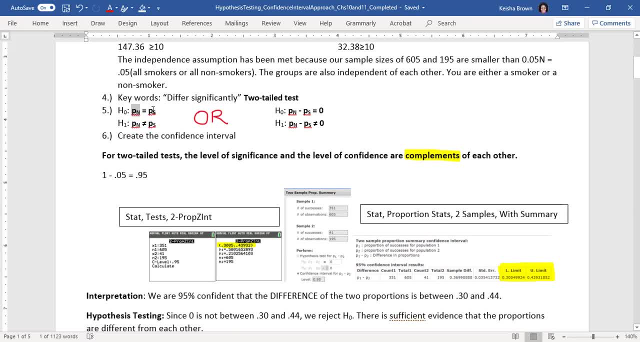 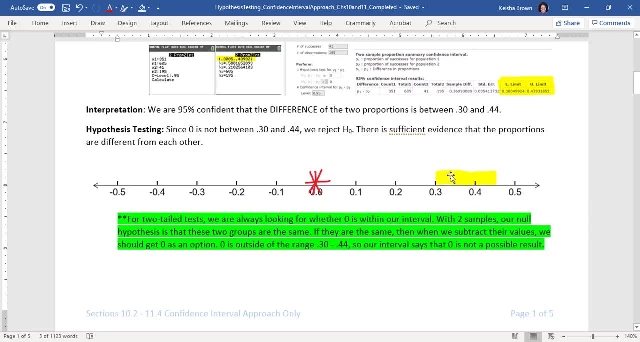 the null hypothesis. Our null hypothesis says that these two groups are equal And if they're equal, when we subtract them we're supposed to get zero. But zero is in between 0.3 and 0.44.. So we're going to reject the null hypothesis. 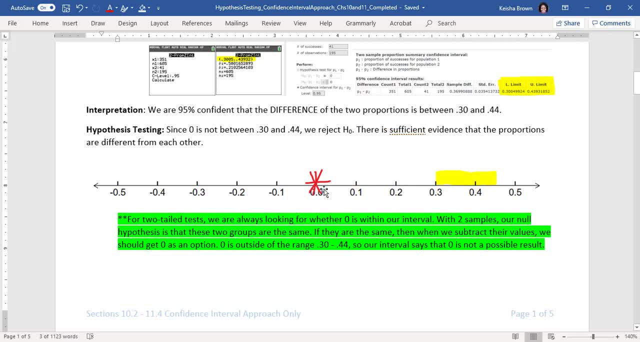 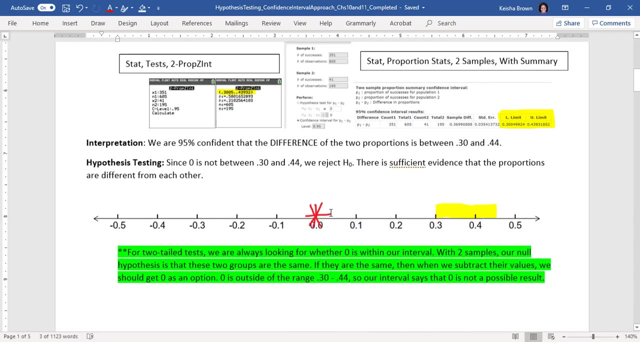 And when we reject, that means there's sufficient evidence, or we can say there's statistically significant evidence, or we can say there is enough evidence that the proportion is different between non-smokers and smokers. We're going to skip over this example. 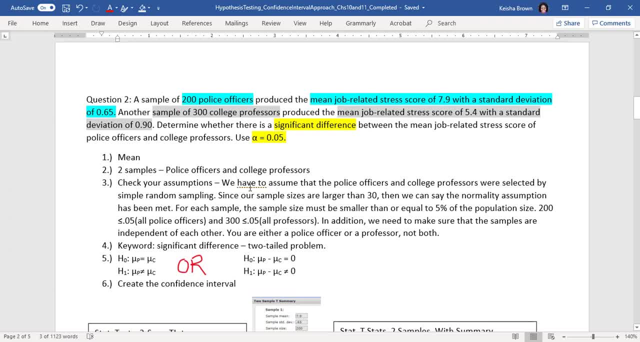 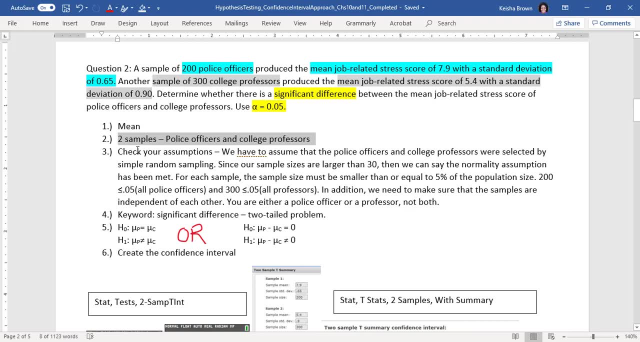 It's a mean problem with two samples. Our approach is the same. You identify your parameters, You identify whether you have one sample or two. You check all of your assumptions, making sure that you look at how was the data selected. is the shape of your distribution normal? are the individual samples independent of? 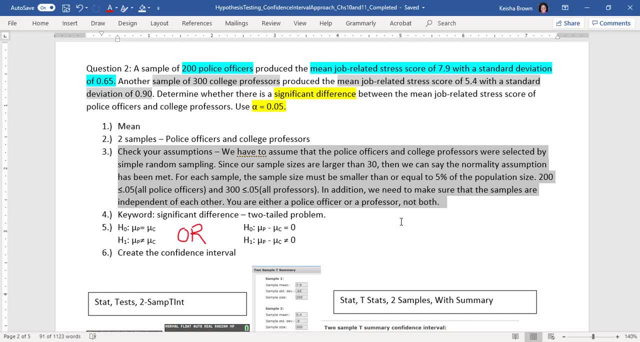 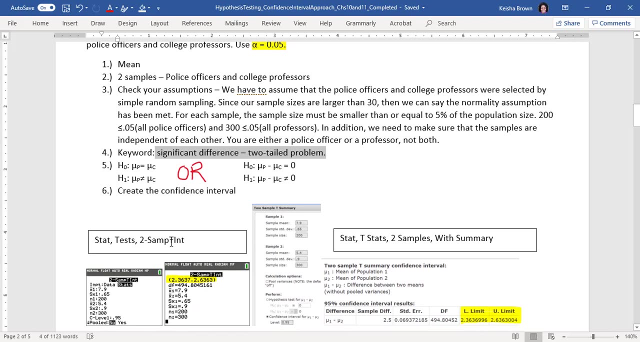 each other and do you have independence within each sample in relation to the population? Two-tail problem. That's the only time that we can do confidence interval approach. You can write your answer two different ways: Calculator- people- you're going under stat test- and 2-samp-t-int. 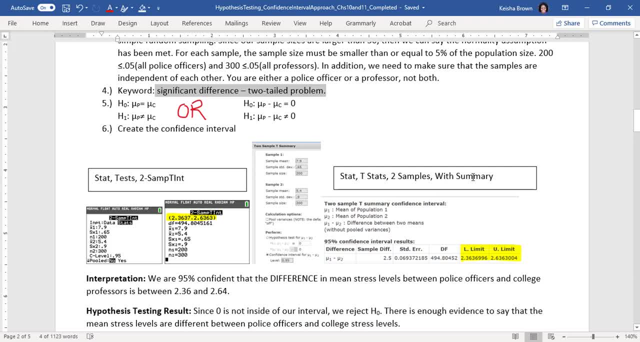 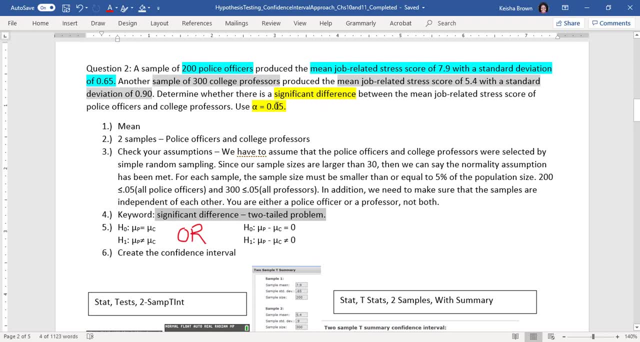 Stat crunch people, you're going under stat t-stats. two samples with summary. Our interpretation: 95%, because alpha is 5%. No, it's not always 5%, We just use it a lot, though. The difference is that we're going to use it a lot. 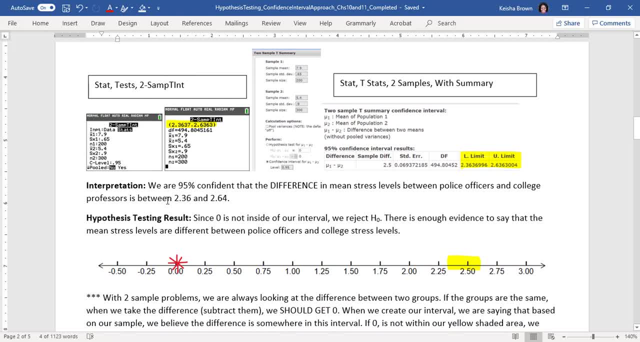 We're going to use it a lot. The difference in stress levels is between 2.36 and 2.64.. Here are where those values fall in number nine: Remember, this interval is created based on your samples. This interval is created based on your samples. 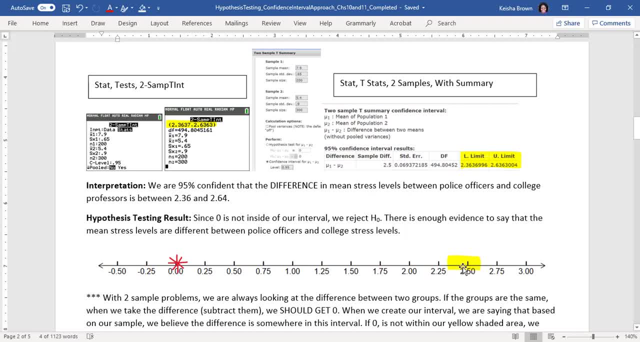 Based on your samples. it says the difference is somewhere over here. In order for us to say that these two groups are the same, zero has to be in the middle of that interval. It has to be somewhere in there. Since it's not, we reject the null hypothesis. 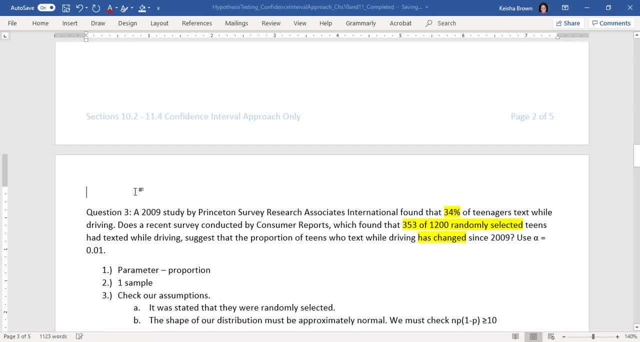 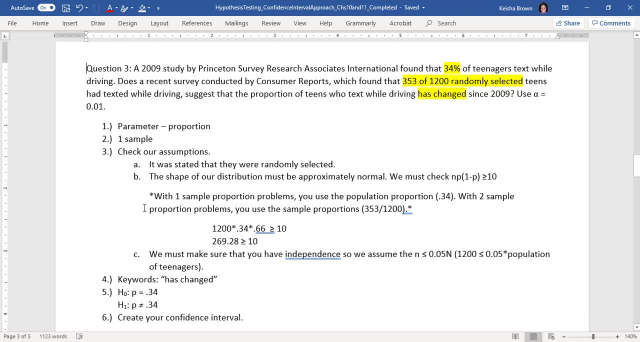 We have question number three. This is our one sample proportion. We know it's a proportion because of that percentage. We also know it's a proportion because you have a number out of another number. It also says proportion here, so that helps. 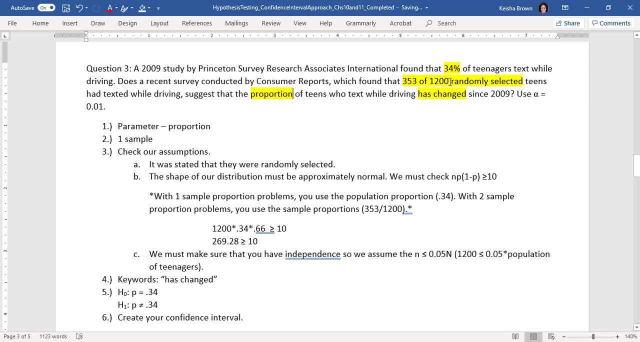 We have one sample. We took one group of 1,200.. Check our assumptions. We took one group of 1,200.. We took one group of 1,200.. We took one group of 1,200.. How did you select your data? 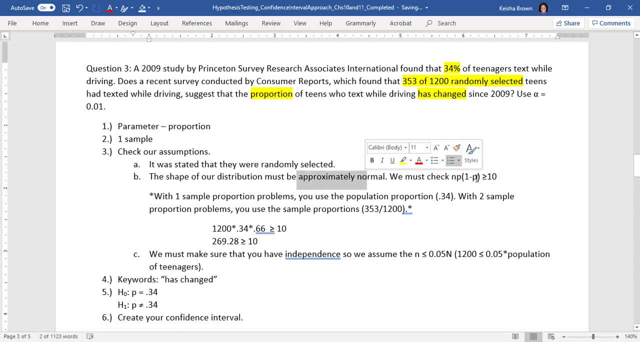 Checking for normality: n times p times 1 minus p has to be greater than or equal to zero. That's our p sub zero. from our null hypothesis, This value we're going to use with one sample is that 0.34. 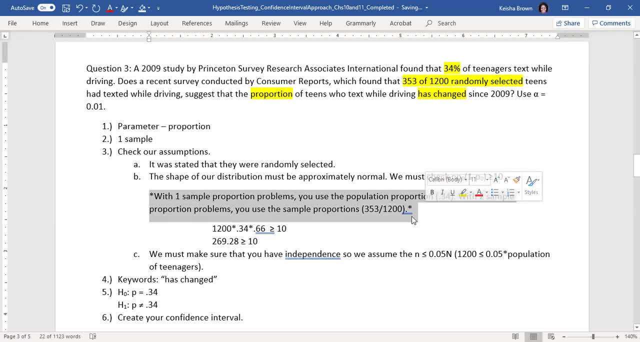 Then there is my note that if you had two samples, you used the sample proportion for each of your groups. When it's one sample, you used the population proportion. We have independence. We want to make sure that our sample size is not too big. 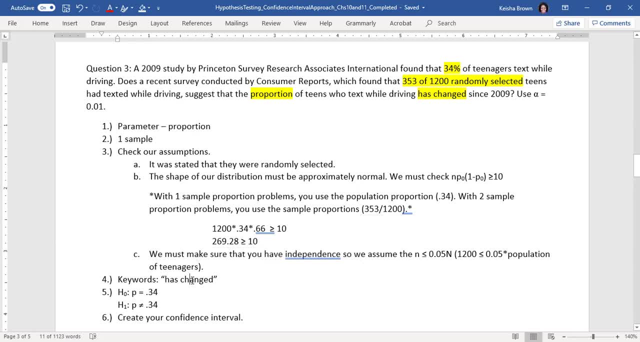 It's smaller than 5% of the population size. Keyword in the problem that lets you know that this is a two-tailed test is that it says: has it changed since 2009.. Null hypothesis is equal to 0.34.. Alternative hypothesis because of the keyword: has changed. 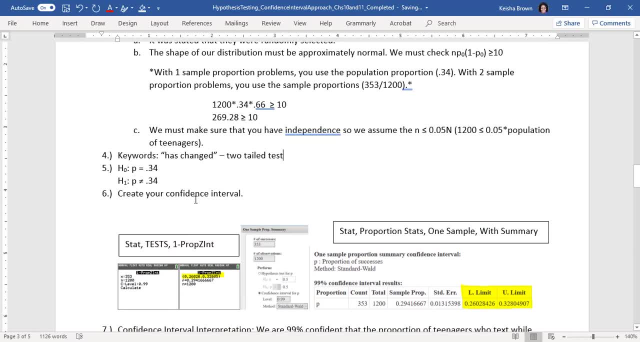 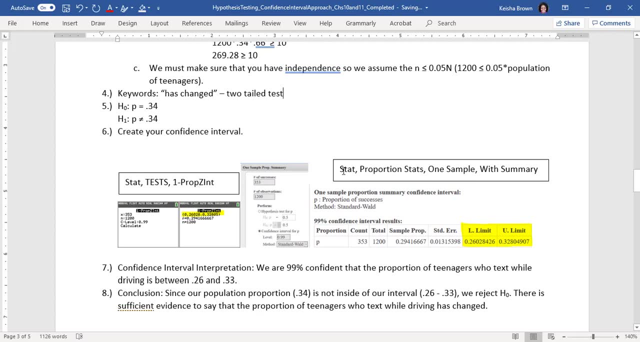 It's not equal to. We create our confidence intervals. calculator: people, stat test. one prop zint stat crunch people, stat proportion stats. one sample with summary: our confidence interval interpretation. What do these range of numbers mean? 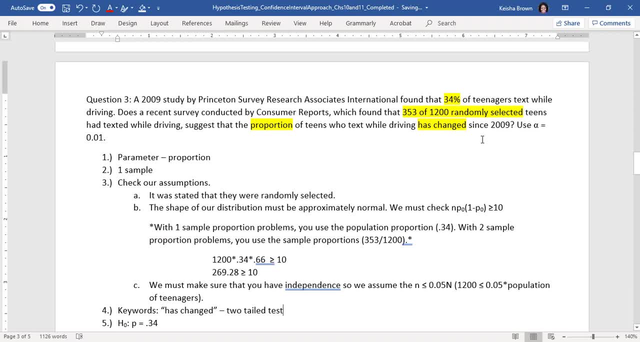 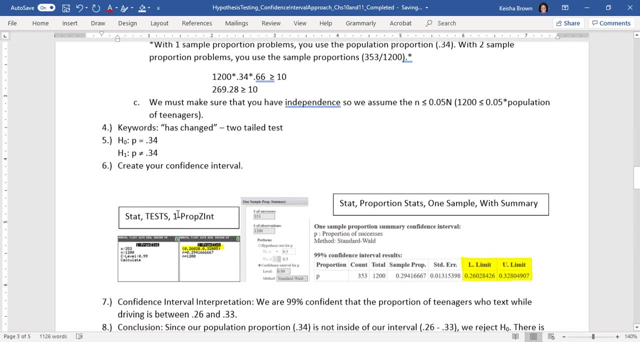 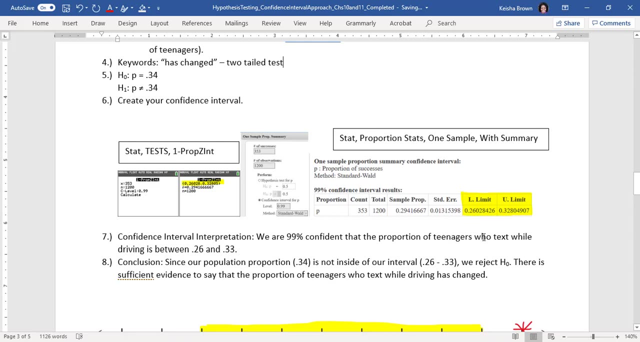 It means that we are 99% confident. Why is that 99%? Because in this problem, alpha is 0.01.. Remember, For two-tailed tests, alpha is the complement of your confidence interval. We're 99% confident that the proportion of teenagers who checks while driving is between. 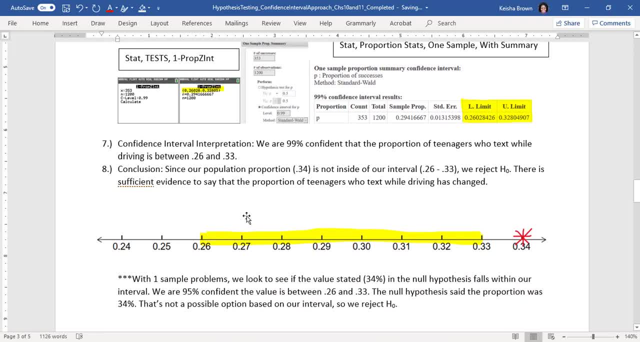 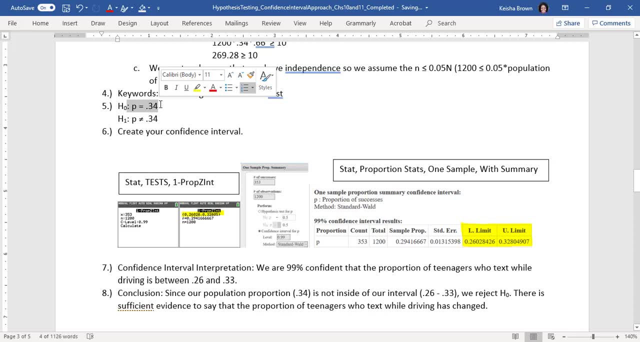 0.26 and 0.33.. For one samples, you're looking for the null hypothesis. For one sample and confidence interval approach, you're looking for the null hypothesis. Is this number fall? Does that number fall? It's a hypothesis. 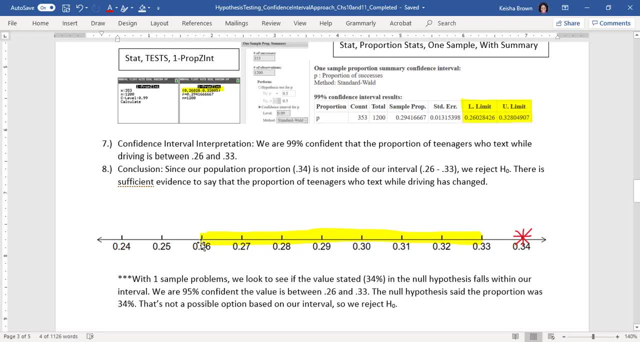 It's not inside of your interval And it does not. Our interval says we think the number is between 0.26 and 0.33.. Null hypothesis says it's 0.34.. Since that's not inside of our interval, we reject the null hypothesis. 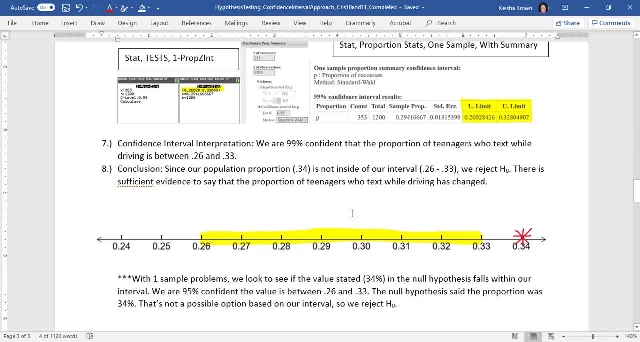 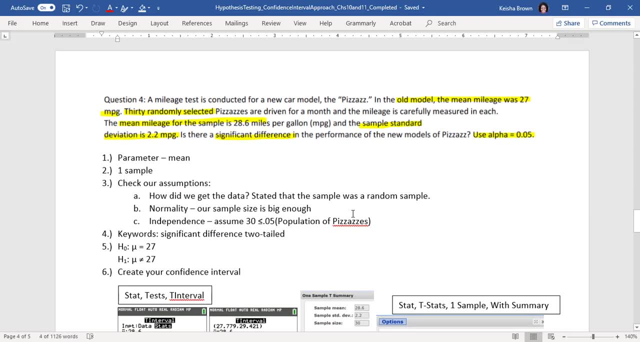 We say that that's not possible. So there is sufficient evidence to say that the proportion has changed. And question number four: A mileage test is conducted for a new car model, the Pizazz. In the old model, the mean mileage test. 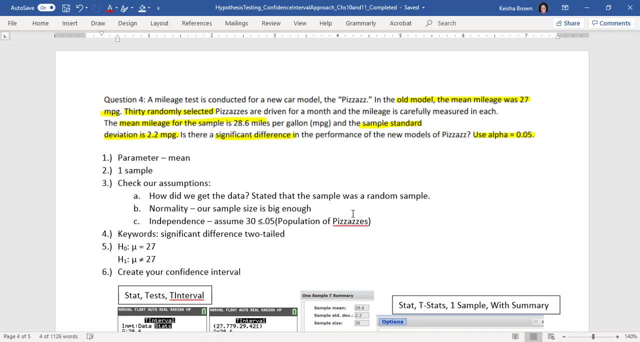 I'm going to do it in the new car model, the Pizazz. The mean mileage was 27 miles per gallon. 30 randomly selected pizzazzes were driven. the mean mileage for your sample- So that's X bar- is 28.6 and your sample standard deviation. 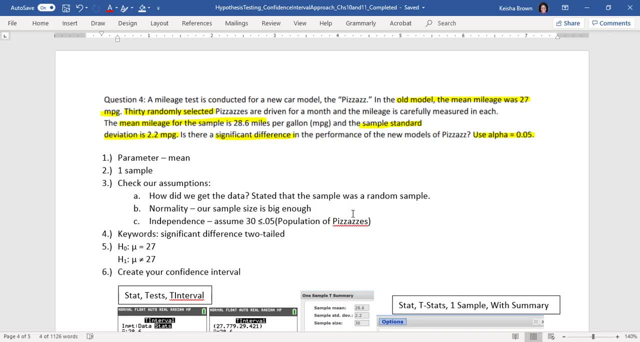 That's s is 2.2.. Is there a significant difference? There's your keywords to let you know. This is a two-tailed test. use alpha equals 0.05. Mean problem because it said: mean You have one sample, you took one group of 30. check your assumptions. How'd you get your data? 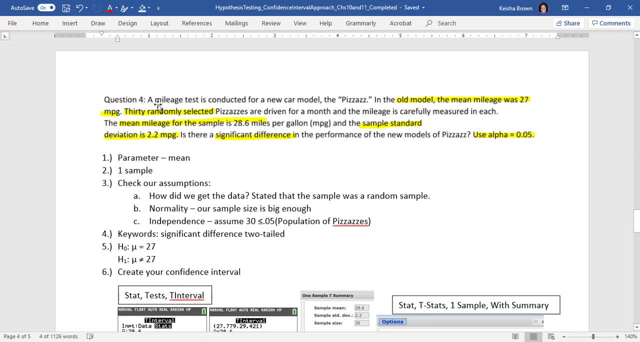 Normality. our sample size is big enough. We have 30 randomly selected pizzazzes and Independence assumption is that our sample size is less than or equal to 5% of the population And we're pretty sure they've made more than 30 cars. 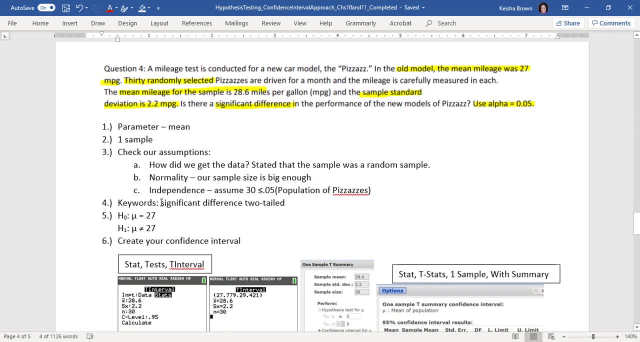 lots more keywords. is there a significant Difference? and that's what lets us know that this is a two-tailed test. our null hypothesis. This is, remember, your old information. So in the old model the mean mileage was 27 miles per gallon. We want to know if there's a significant difference. have they made enough improvements to say there's improved gas mileage? 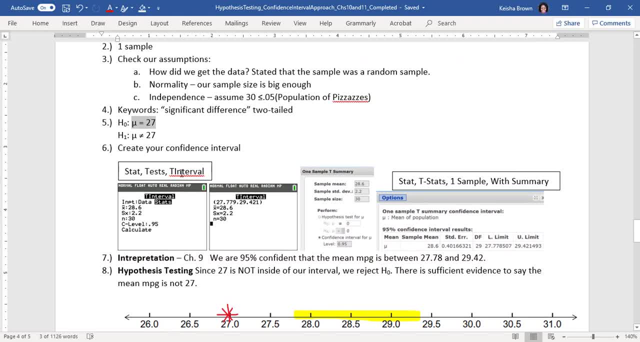 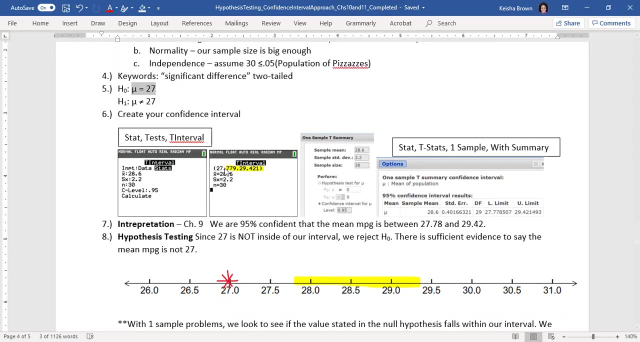 Calculator: people stat tests T interval. when you have one sample stat crunch, people stat T-stats, one sample with summary, you have your Confidence intervals that have been created here and here How we interpret these values. We are 95% confident that the mean miles per gallon is between: 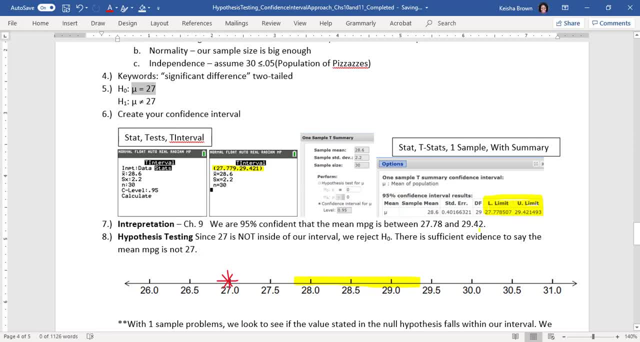 27.78 and 29.42, and once again, this is based upon our sample of 30, So do we have enough proof to say that It's changed? Well, the mean was 27. That's what it said last in the old models. now, 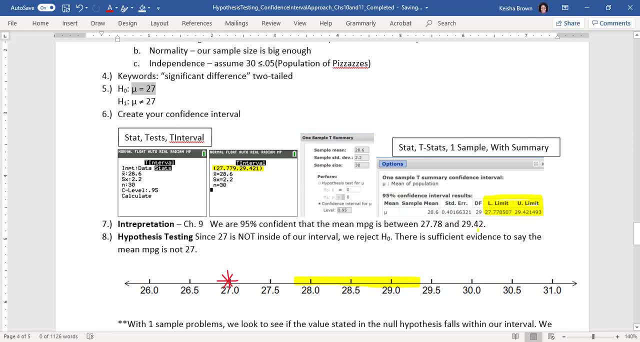 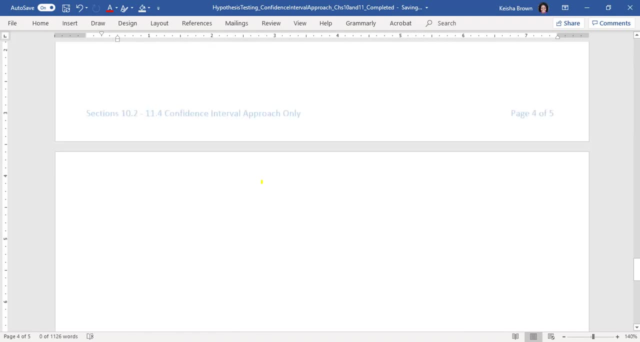 We're saying our mean is between 27.78 and 29.42. So since our null hypothesis value is not inside of our interval, we reject the null hypothesis. We say that the mean has changed. we have sufficient evidence. That is our review of section. well, 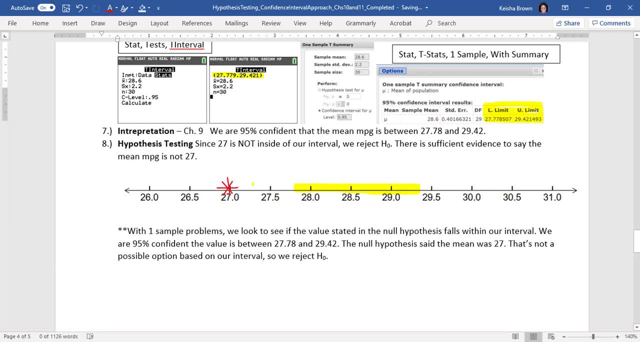 Evidence interval approach covering chapter 10, which was on one samples, and chapter 11, on two samples. Send me an email if you have any questions.